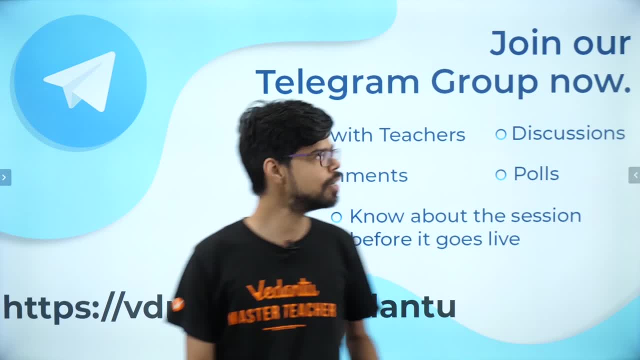 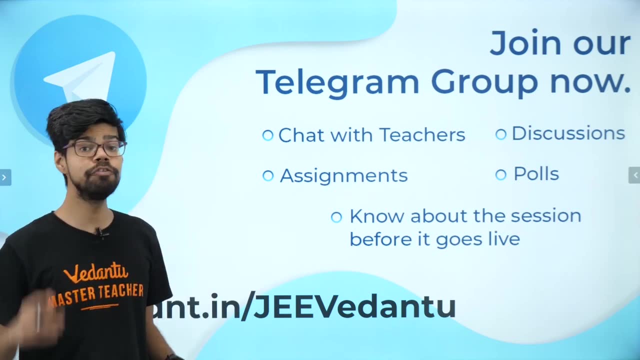 but has some awesome features which we try to use. So on this channel you can have, you can chat with us, the teachers faculty, you can have discussions, you can solve your doubts, you can post your doubts. We will also be posting some assignments. 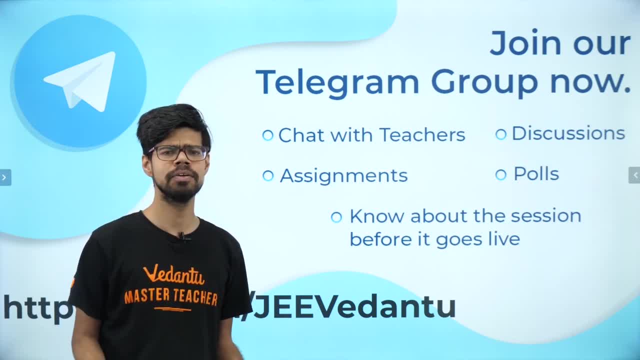 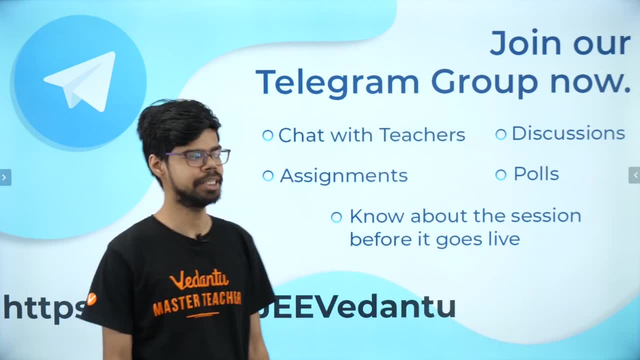 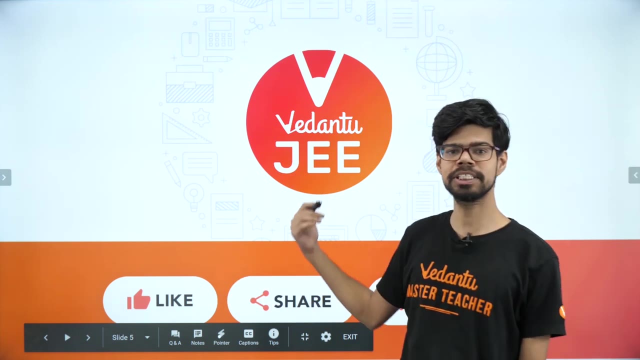 So that you can practice and all the interactions with the faculty and among each other. So it is very helpful and it will help you a lot while preparing for your KPBY examinations, which is in November, Okay, next. So also please share, like and subscribe the channel as it grows and you get. 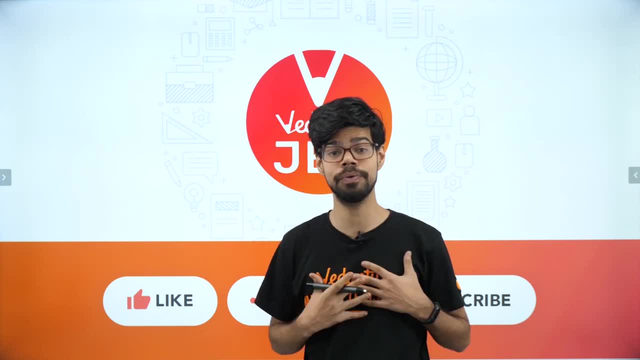 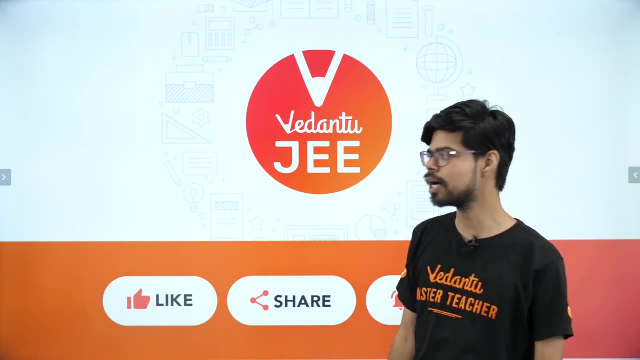 more and more people, the community grows and it helps each and everybody of you. Okay, and that is also very important, So please hit the like button and subscribe to the channel. So, before wasting more time, start with the first question. this is the first question. read it and, if you, 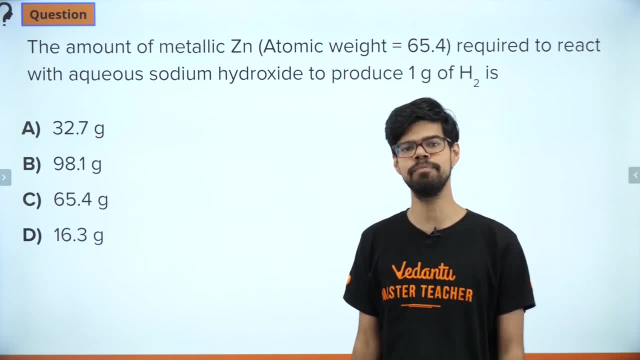 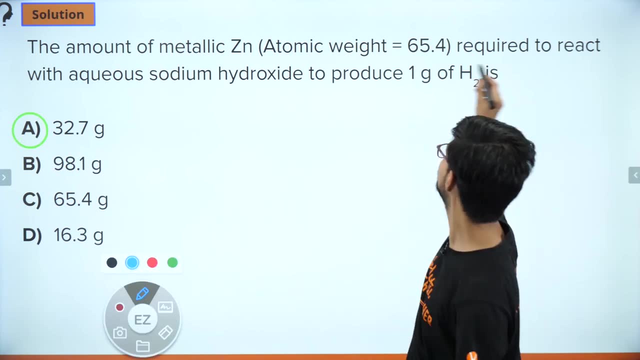 want to try it. pause the video right here and attempt it. okay. so the question is: we start with a simple one. the question is: we have a metal zinc and it is treated with sodium hydroxide. okay, the metal zinc is treated with sodium hydroxide and alkali and hydrogen gas is produced as a result, and you have to. calculate how much of zinc is required to produce exactly one gram of hydrogen. okay, so for that we do the general problem solution. so if we first write the balanced chemical equation, which is this: zinc plus an image gives hydrogen and sodium. zincate with the formula is written ice like. 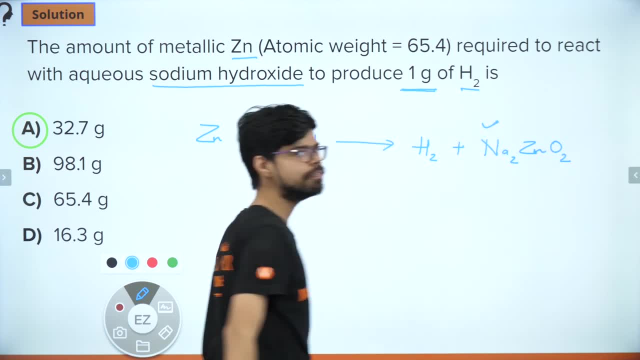 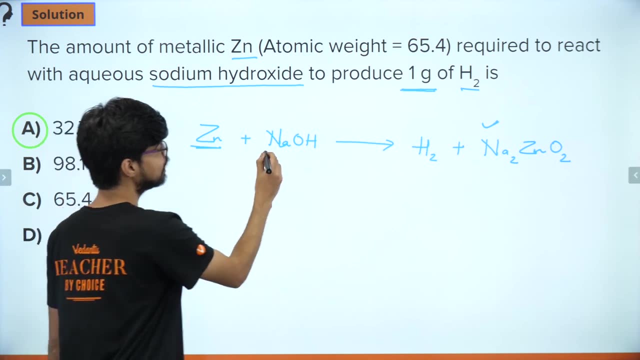 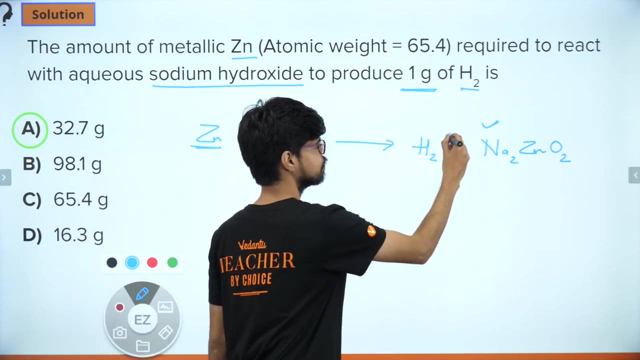 this. so this is a tricky part. this is a reaction with. it is not that common but extremely important. so zinc metal reacts with alkali. it can be any alkali here it is any which you can be. calcium hydroxide, it can be anything which produces hydrogen gas. and this other product is sodium zincate. I'll write the. 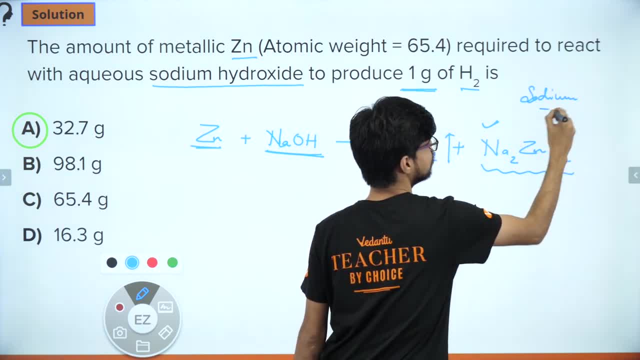 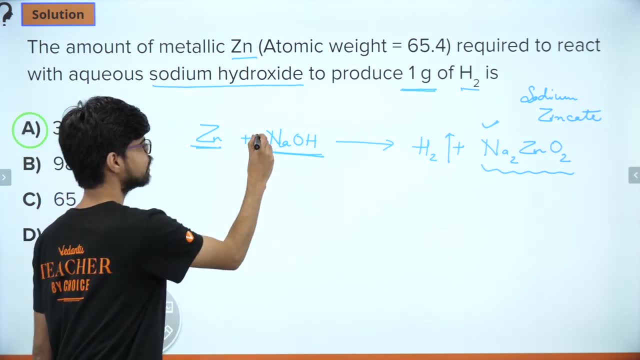 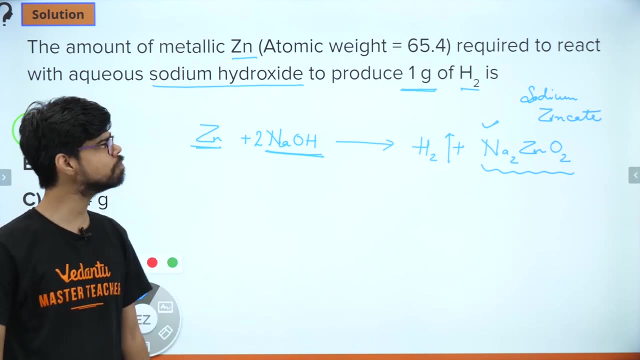 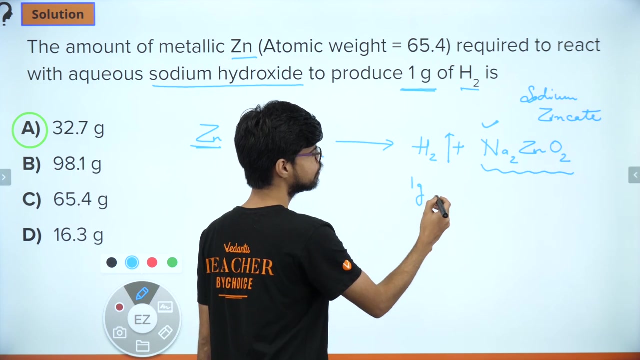 non name down here. okay, so now next step is balance it, and we can do that by just adding a 2 here, and this is the balance equation. rest. what is next? any mole concept problem: first convert the masses given to moles. we can always solve in moles, so one gram. I just solve it right here as 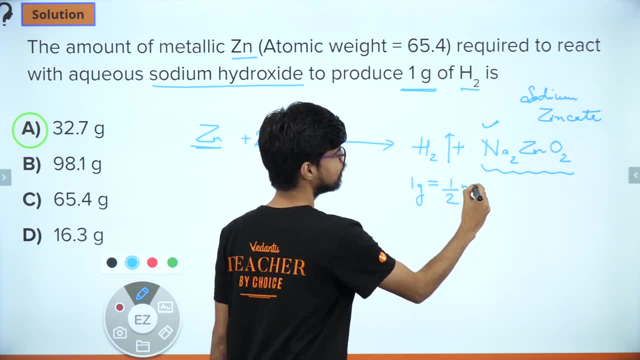 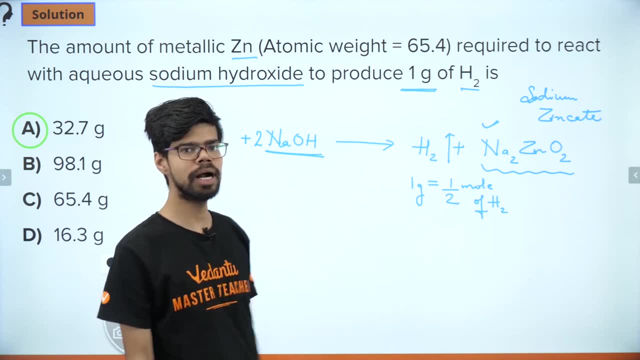 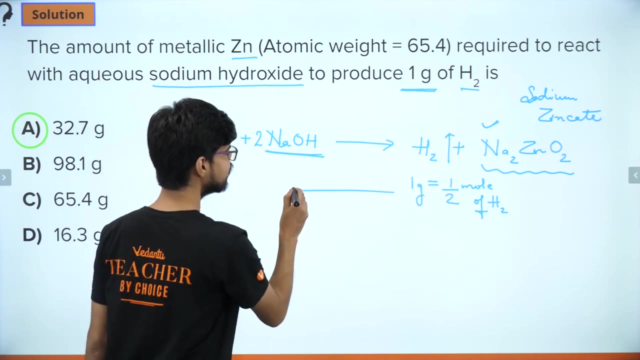 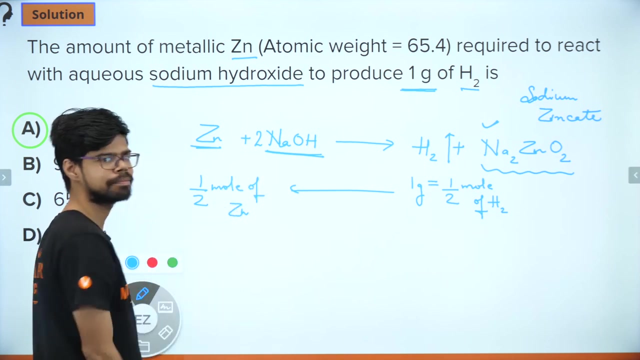 you can do it. it is half mole of hydrogen, right, that is simple. so half mole of hydrogen is required, and we can see from the equation that for one mole of zinc you get one mole of hydrogen. so from here we I can directly say half mole of zinc will be required. right, half mole of zinc is required. 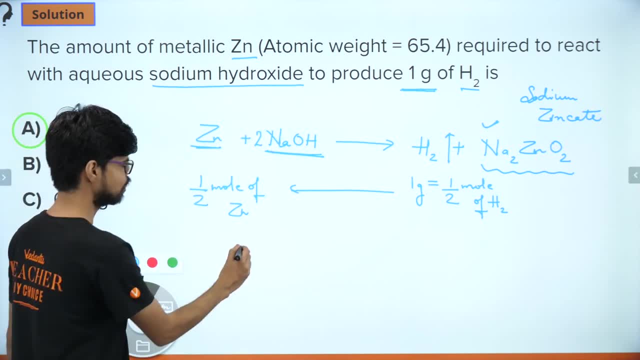 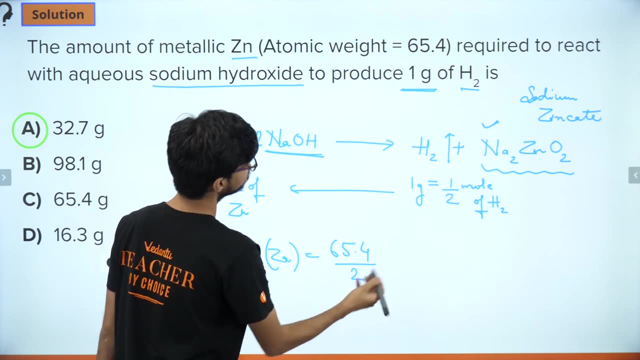 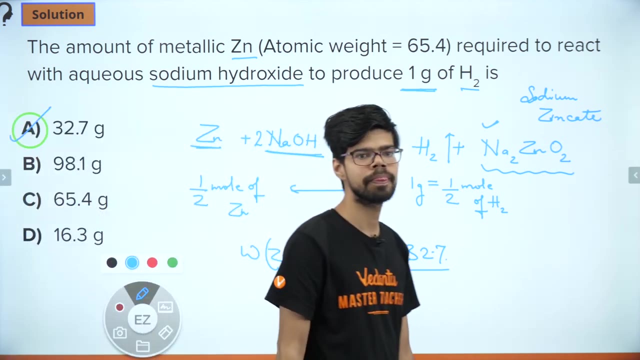 atomic weight is giving, you can calculate the mass. so mass of zinc will be half of 65.4, whatever the mass is, and that comes out to be 32.7. let's check the answer and we have it here. okay, Easy one, just go through it. you write the equation. you have to know the reaction. that 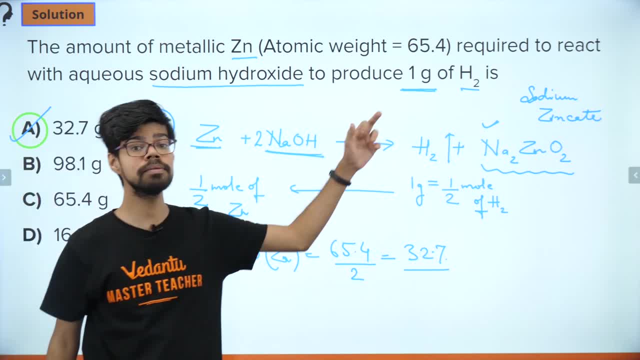 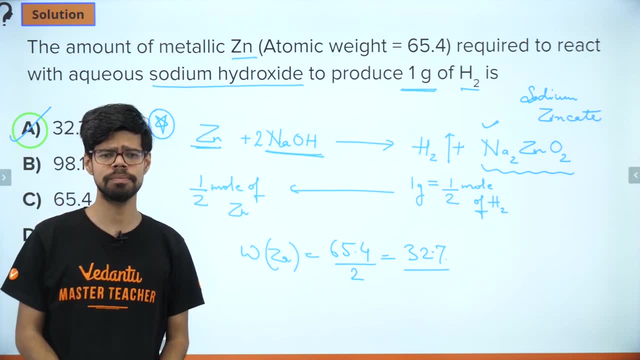 is important, then solve it. convert mass to moles, then back from moles to mass. That is the basic, general point of a mole concept problem. So it might seem easy, but I will tell you something else about this problem. 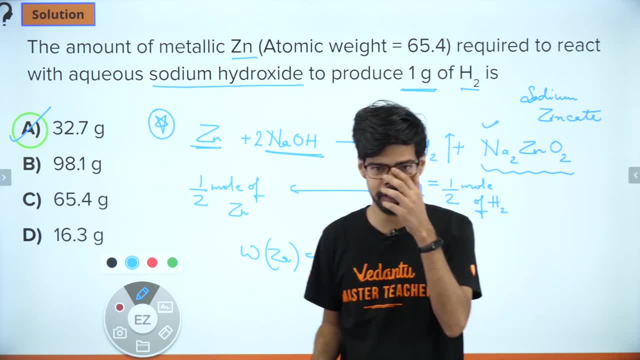 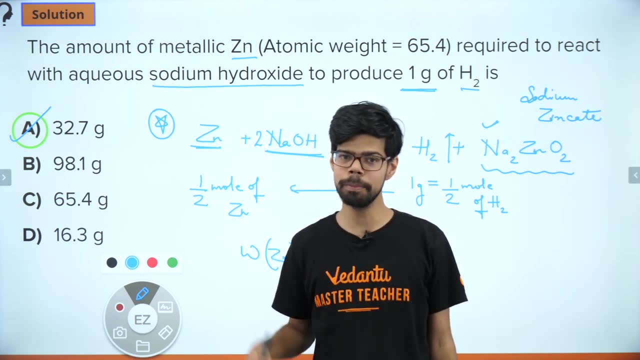 This is a previous year KBPEI questions. All the questions which I am taking today are from previous year papers. So all of these questions have appeared one or the other years previously. So if they appear easy, it is very good. if they do not, if you even get to that level. 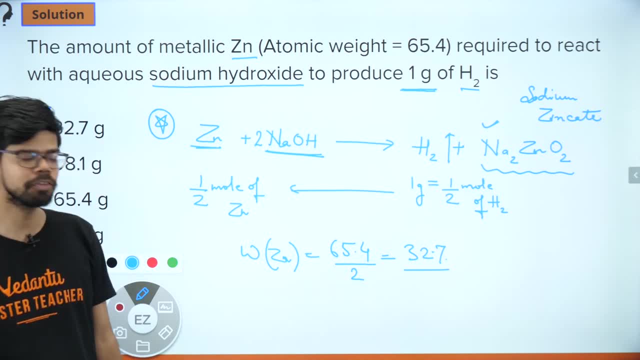 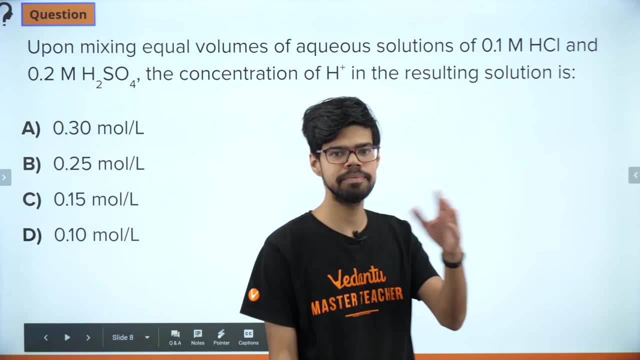 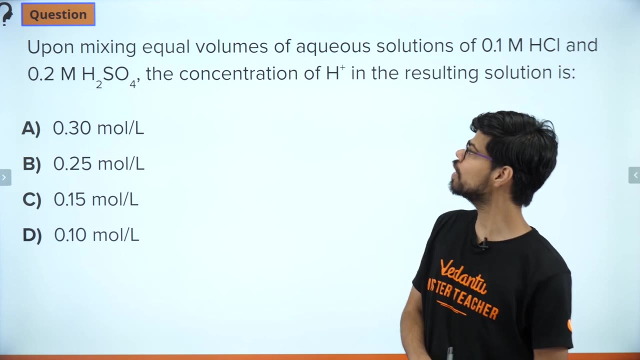 it is very relevant for the KBPEI exam. If you found it easy, let us do the next one. This is the next question. Again, same thing. pause the video. try it, then stop. So this is on the topic of molarity and concentrations. 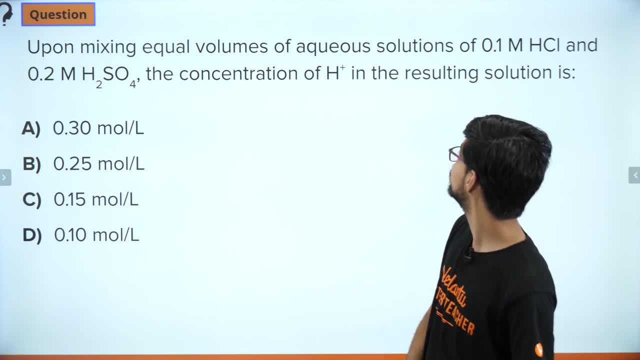 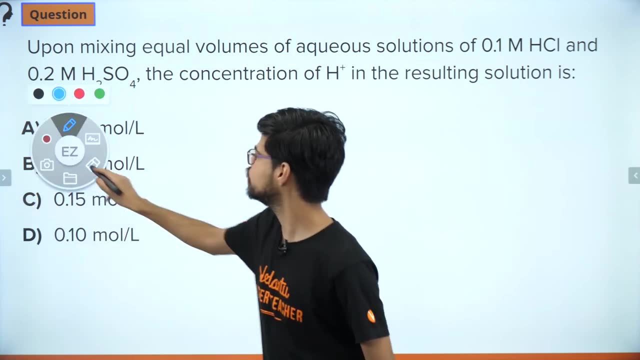 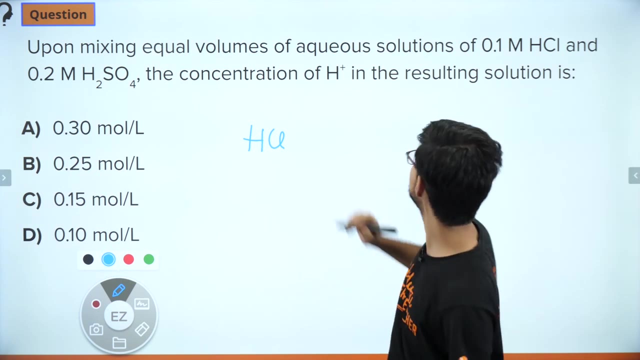 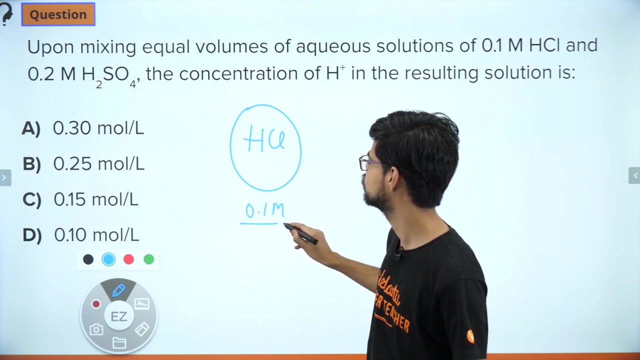 Again and mixing. so what we have done, we have got here, is we have an HCL solution. Okay, so we have an HCL solution. I will just remove this. So such questions I like to do, try grammatically. so we have an HCL solution which is 0.1 molar. 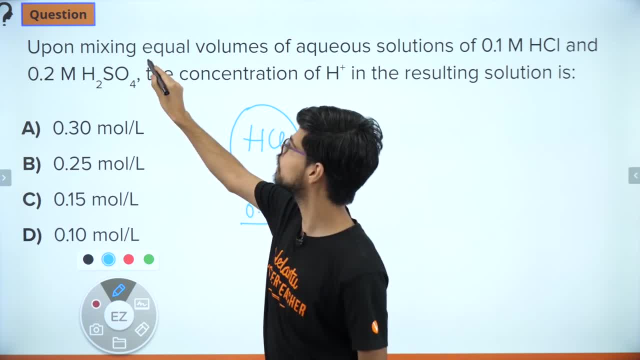 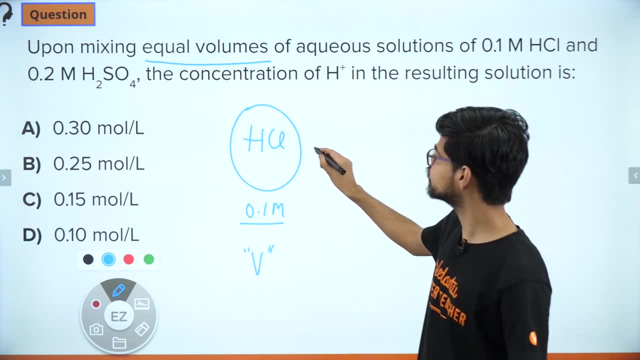 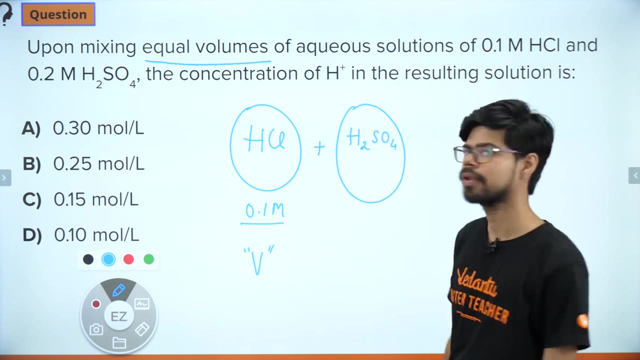 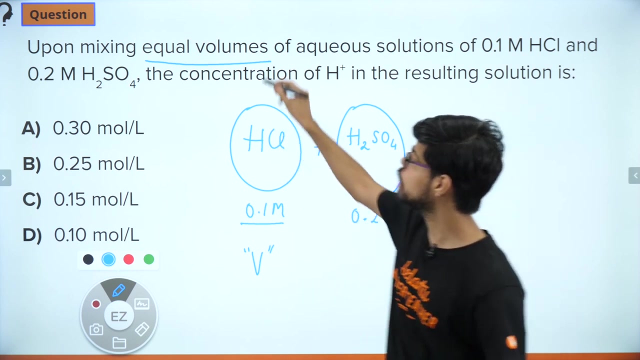 Okay, and the volume is not given. and it is given that the volumes are equal. So let us just say: the volume is some V, Okay, and we are mixing it with an H2SO4 solution- Okay, and the molarity is 0.2 molar. and because equal volumes are given, we can just write: 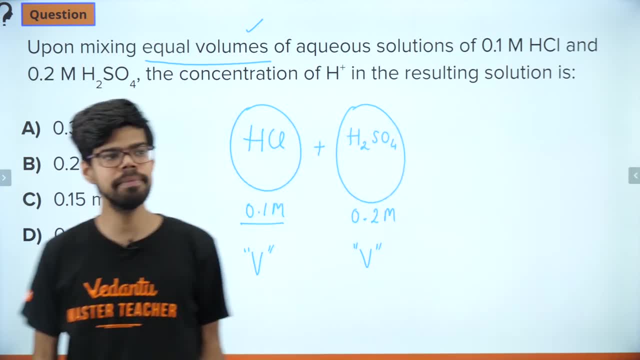 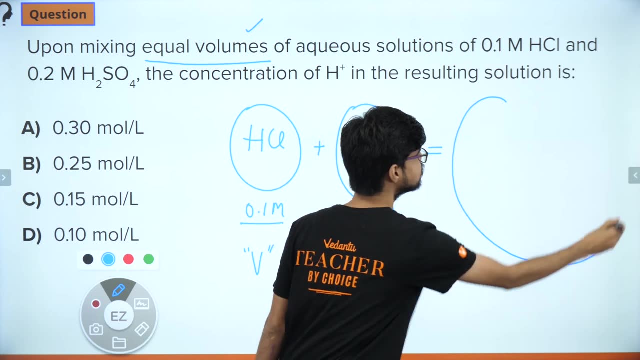 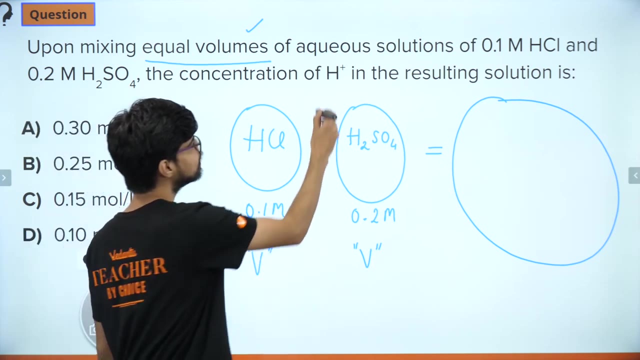 it again: V. Now their solutions are mixed and we have to find the new molarity Okay Of the resulting solutions. So solutions are mixed, so I can add a positive plus sign here and we get a mixture of it, And what is required is we have to find the H plus concentration in the solution. 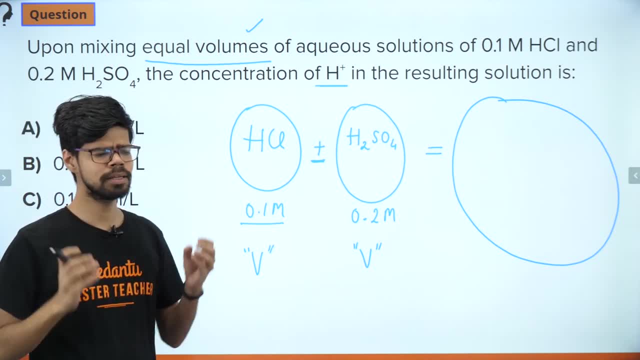 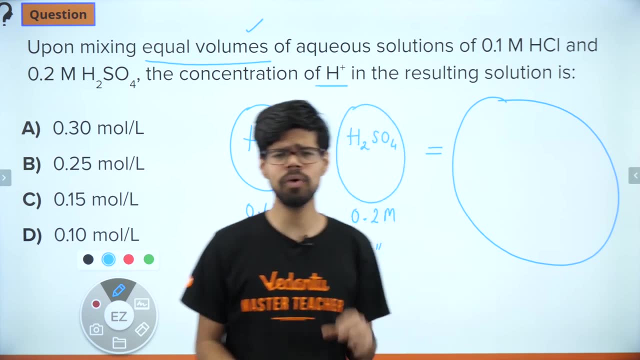 So this is again very simple if you think about it in very basic manner. Many people get confused here. it is pretty simple, So what you have to do is just think about S plus So H plus concentration here is 0.1 molar. 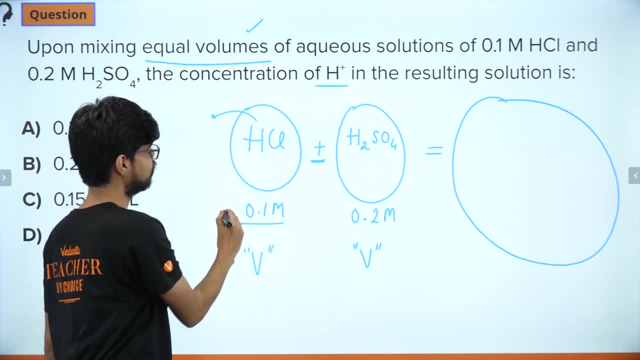 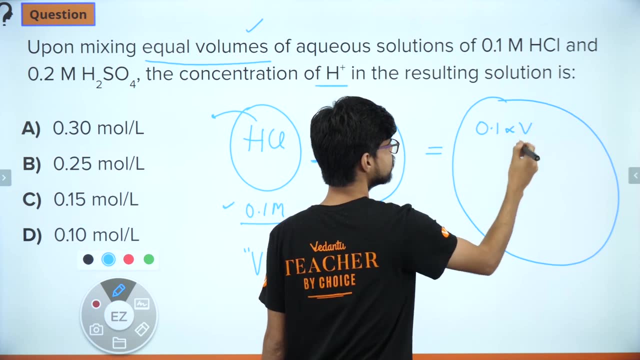 Okay, 0.1 molar, Right, So I can say 0.1 into V. So this is moles of H plus. We are trying to write moles of H plus because the molarity will be moles of H plus upon. 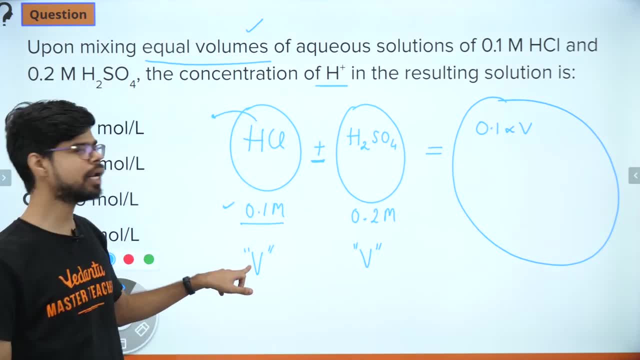 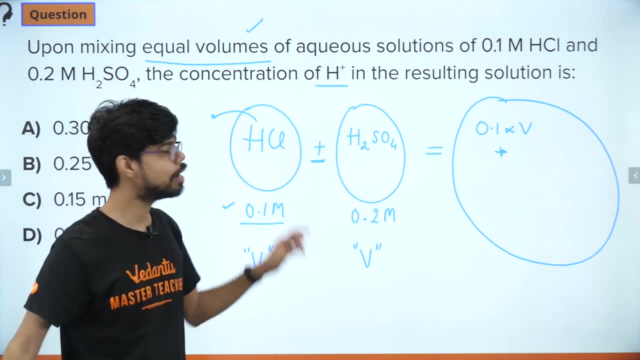 the total volume. So moles of H plus will be 0.1 molar into V Plus. we will also have H plus from this solution, And for 1 H2SO4, you have 2 H plus, Right. 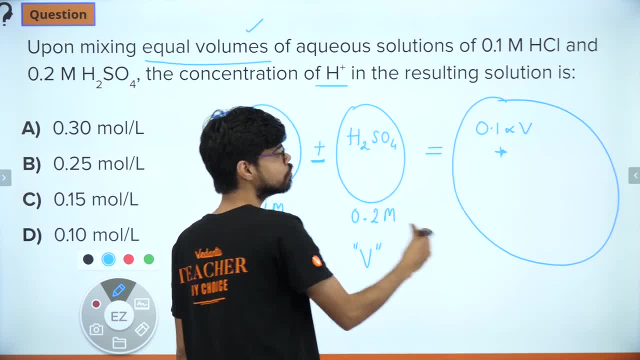 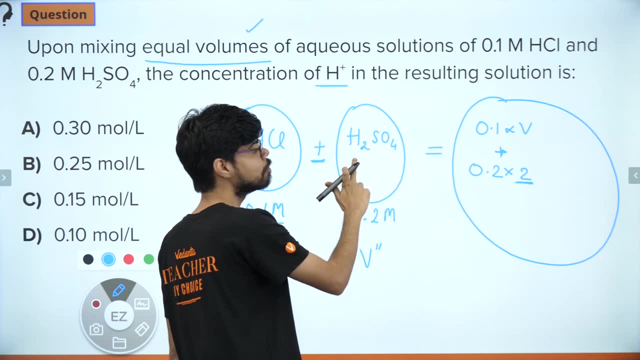 So the concentration of H plus, your moles of H plus from H2SO4 will be 0.2 into 2.. And this 2 is why? Because 1 mole gives you 2 H plus into V. So what is this? 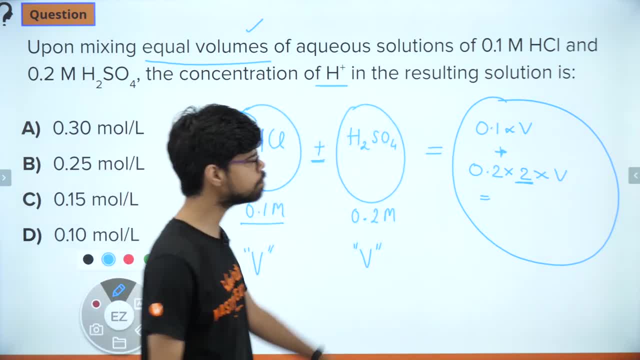 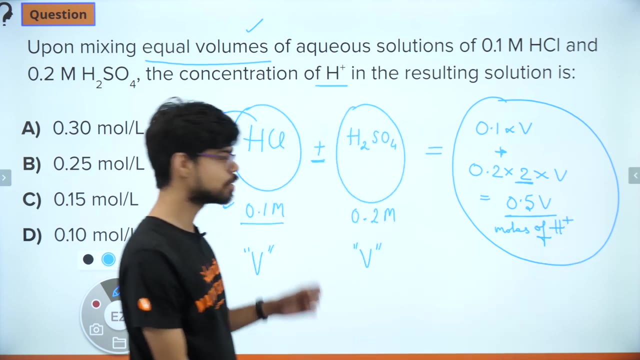 This is moles of H plus. in the solution We can sum it up: We will get 0.5, I guess V. Now this is moles of H plus. Let me write it down: Okay, So that's our moles of H plus into 2.. 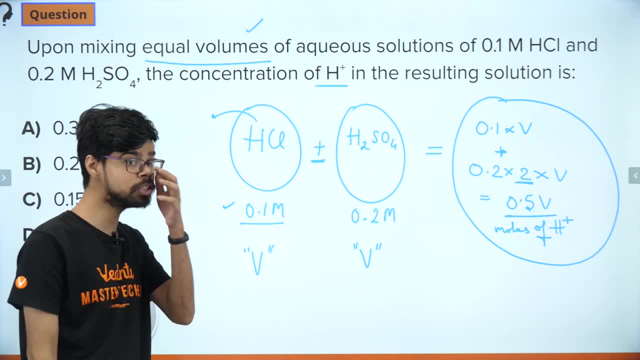 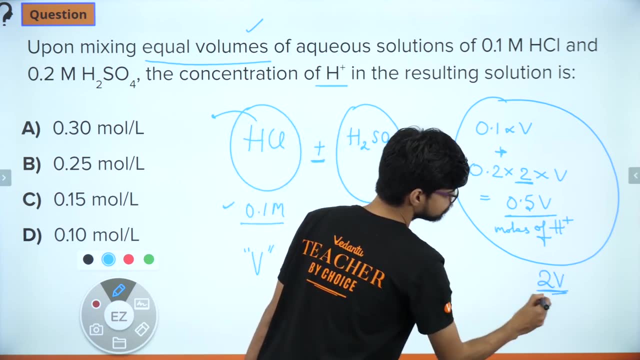 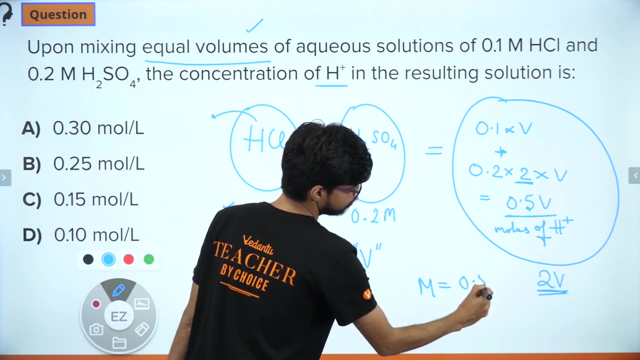 So that's M2 are the moles of H plus, So we will be using as the moles of H plus. Remember last time I explained about H plus is 1V and this M1 is 2 V plus. In due course we can write it down from here. 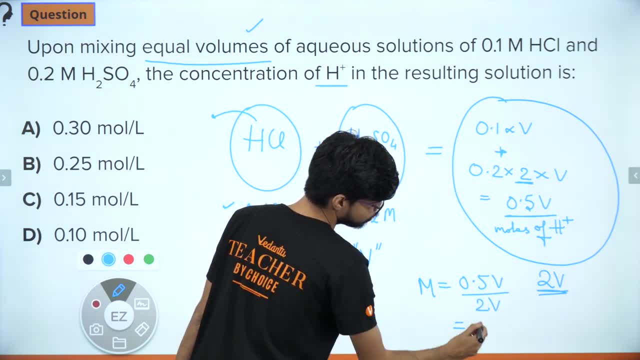 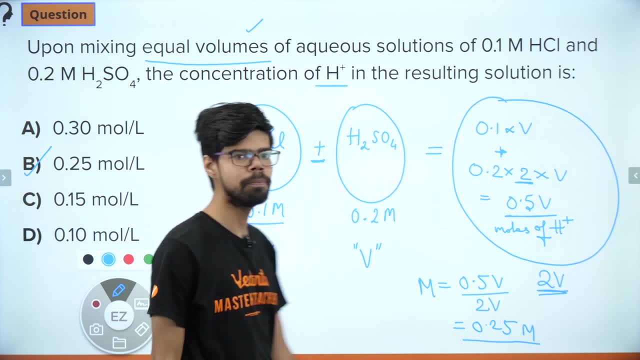 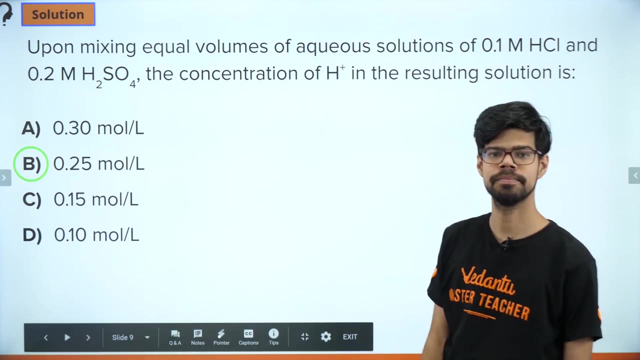 Yes. Now to the, the mole of H and 2, I am using 1,, 2, and 2.. Okay, So the answer is B. I hope most of you would have gotten it correctly. Let's confirm it. So answer is B, Simple. So, while mixing- again, this is a second type of problem, What you have. 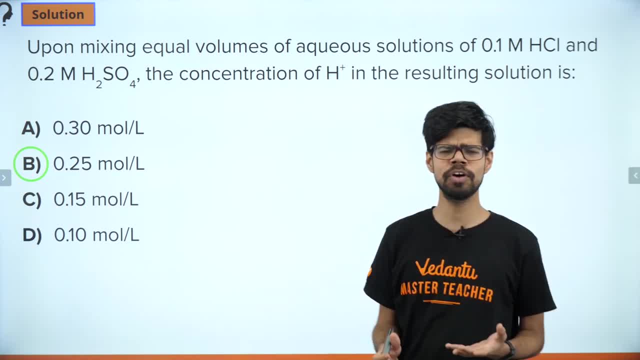 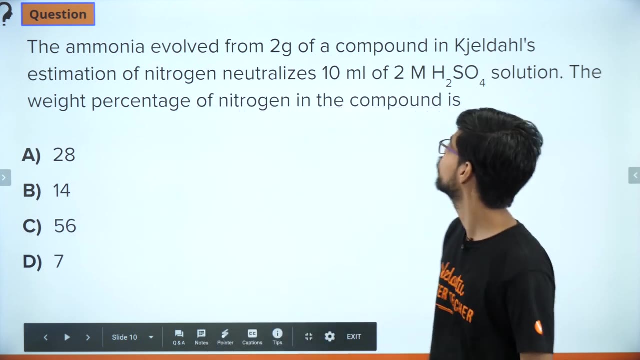 to keep in mind: don't go after formulas, No standard formulas, They don't mean anything. Think about it. simply Just add the moles and add the volume. Divide it. You get a mixture problem. Okay, Next. So this is the third problem. So read it through. So what does it say? It says we have 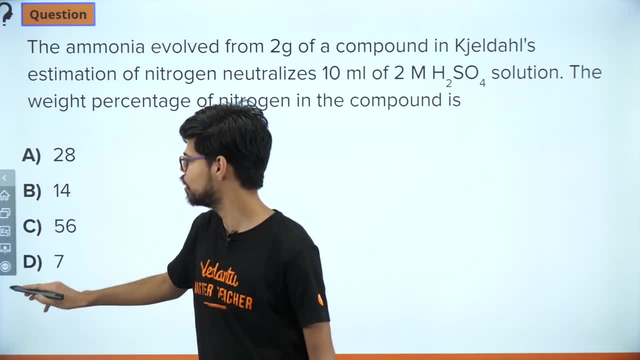 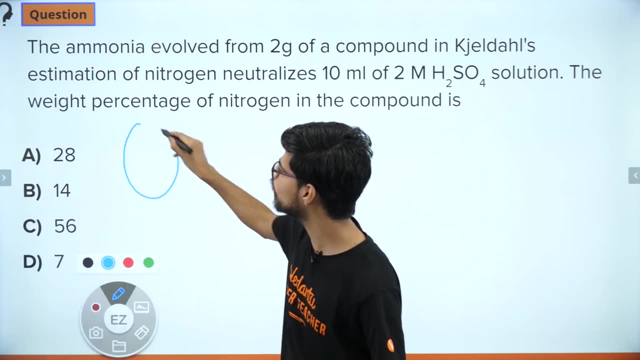 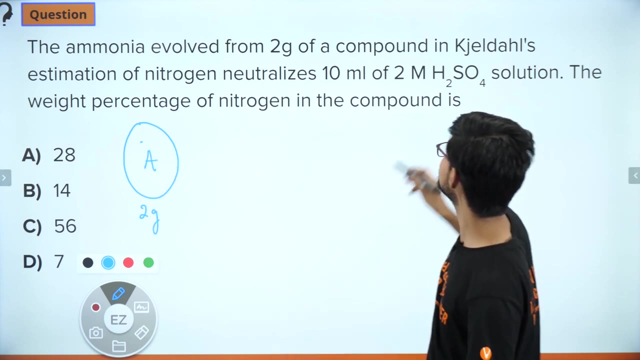 a compound. Again, the best way to visualize the problems is try to draw it in a diagram. So we have two grams of something. We don't know what It is. a compound? Let's say A Okay, And it says A. 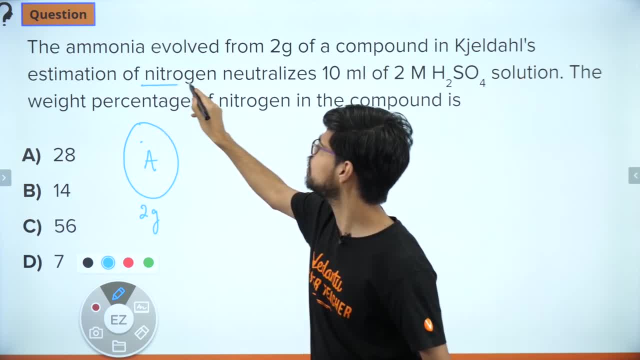 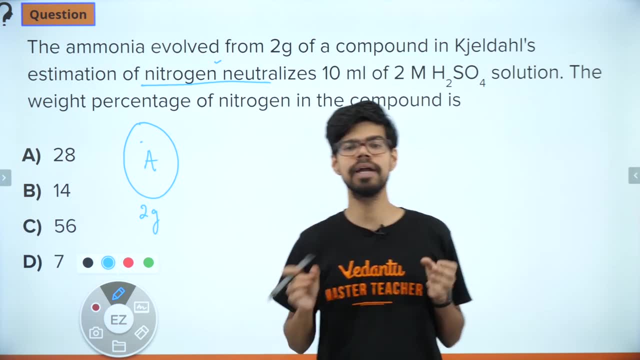 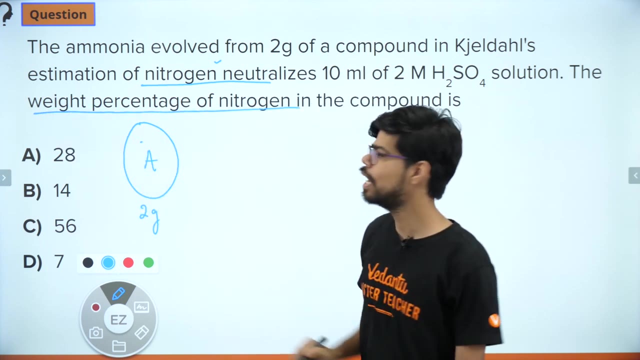 Something, something. Estimation of nitrogen. So what are we trying to do here? We are trying to find the amount of nitrogen in the compound in terms of percentage, The weight percent of nitrogen. we have to find And this is done by Jeldahl's method. So Jeldahl's process is a 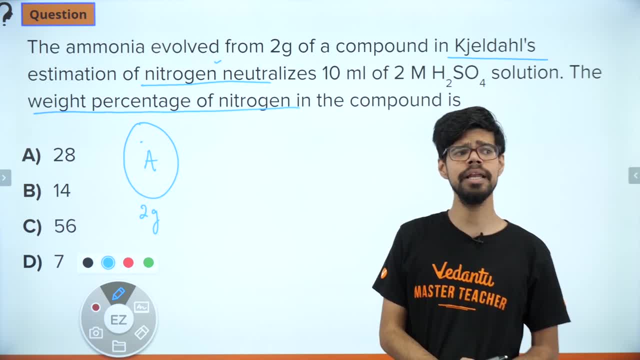 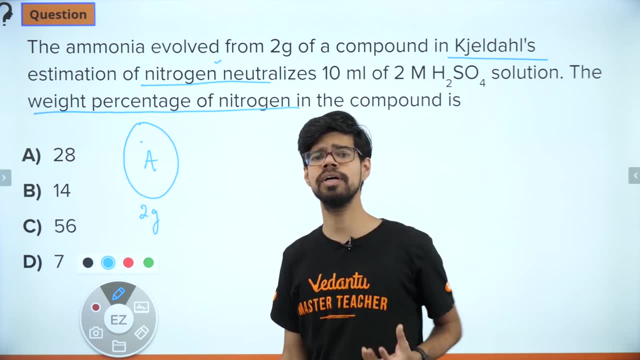 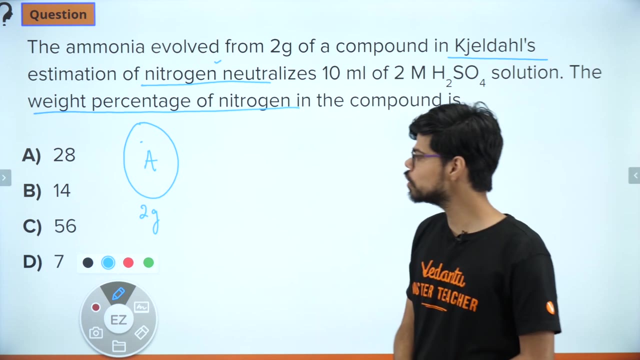 process of finding out the amount of nitrogen in a compound. Okay, In terms of percentage, It is a standard method. You will study about it in your plus one organic chemistry. Okay, We don't know that, But we don't care. We just have to solve a mole concept point of view. Okay, So how do we go? 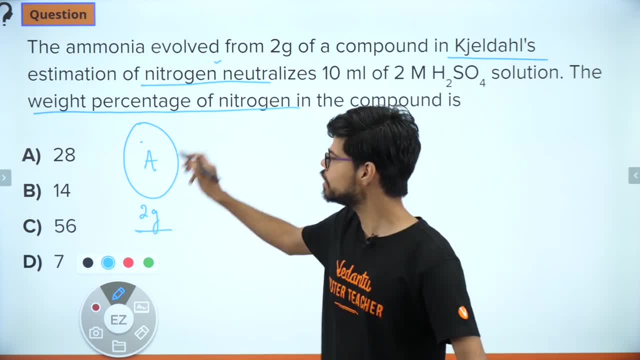 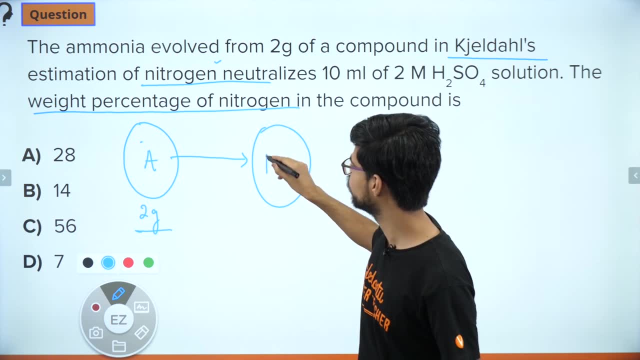 about it. So the general idea is: we do something with it. We don't really care what, And what happens is all of the nitrogen is converted into ammonia. So all you need to know about Jeldahl's method is all of the nitrogen in the compound. 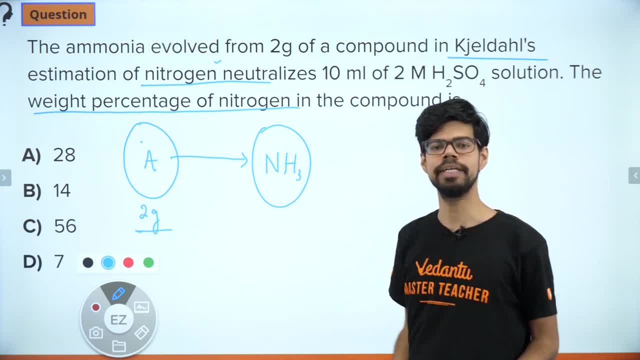 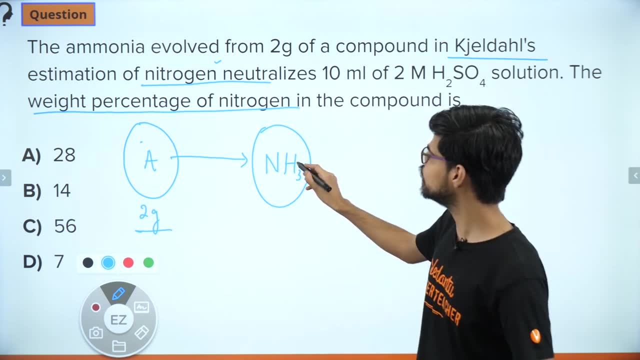 It has some nitrogen. it is converted into ammonia, all of it, okay, and then we measure the amount of nitrogen. that is the method. so what we do then this is a base, and we neutralize it with what acid? so we use 10 ml of 0, not 0. it's 2 molar H2SO4. okay, so we can. 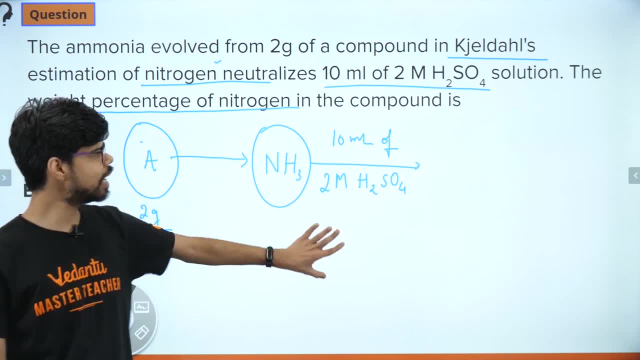 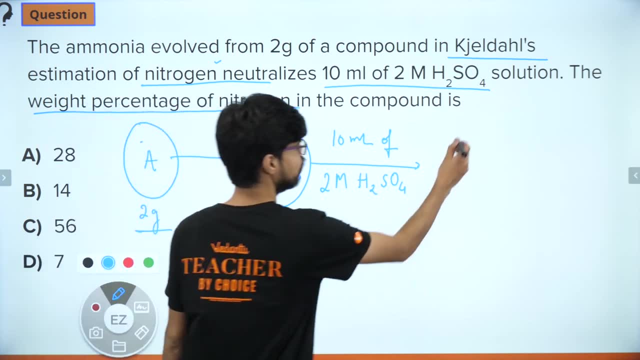 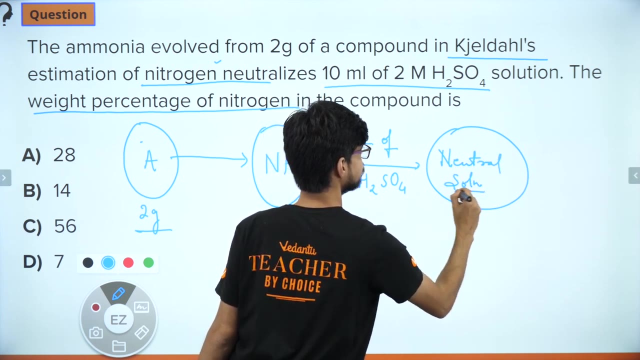 use the equivalent concept for doing this titration. so, basically, why it is being done. you have to understand it. to measure the amount of ammonia, we measure the amount of acid which is needed to neutralize it so we get a final neutral solution. okay, so we can do it by equivalent concept. so number, amount of. 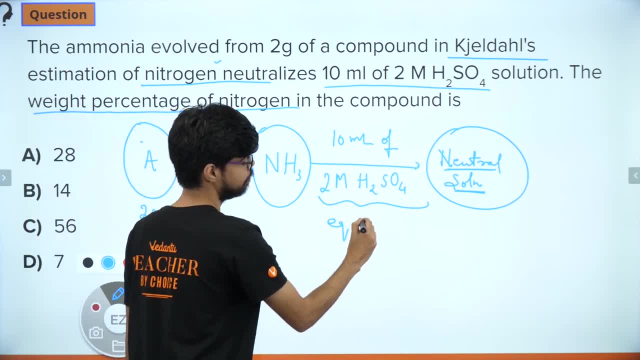 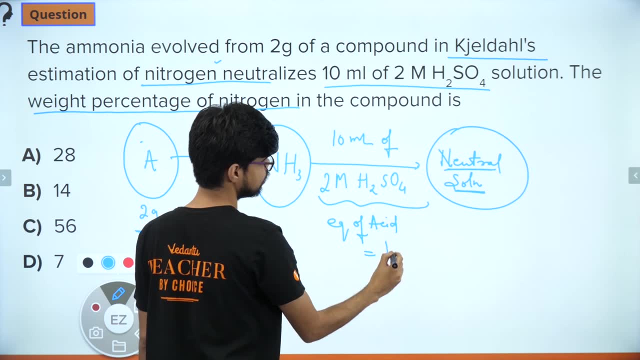 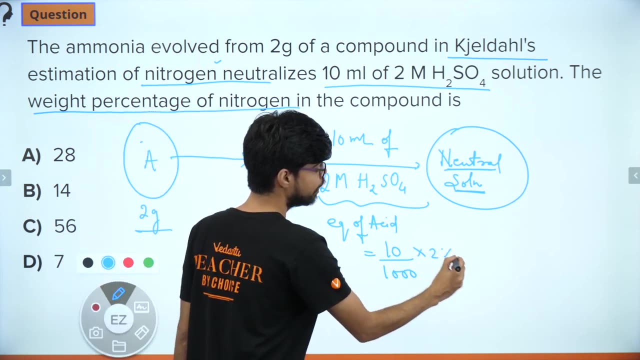 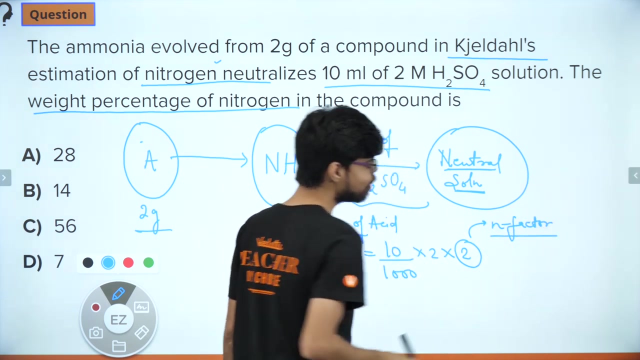 equivalence of acid will be what? 10 ml, so it's 10 by thousand, because we do it in liters, into 2, which is the molarity, and into 2. why this 2 here? this is the n factor for H2SO4, so don't forget this. so we are. what is equivalence? equivalence is basically we. 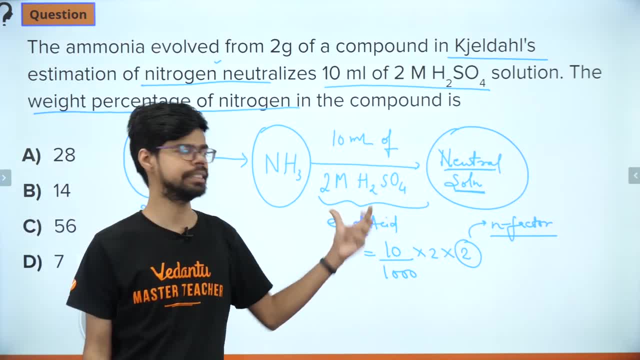 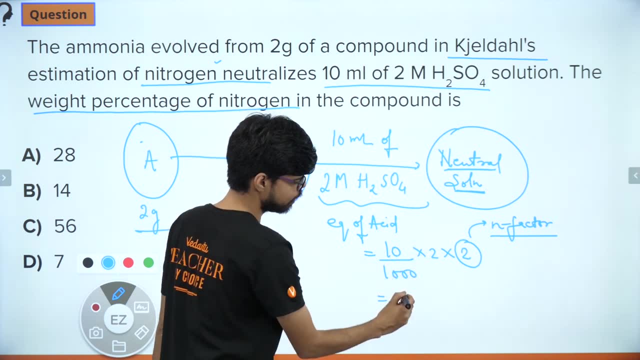 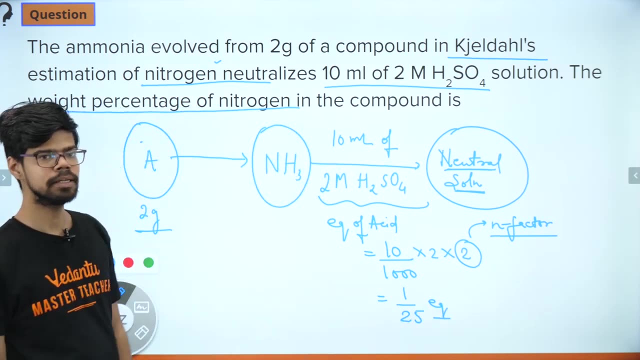 are calculating the amount or moles of H plus from this acid. it will be given by this. okay, you can try and solve it, but it doesn't really matter. so we will get something around 1 by 25 equivalence. now this is acid, and, but? and how does? acid-base titration work. the amount of equivalence of acid is always equal to the amount of equivalence of ammonia. okay, so from here I can directly say we will have 1 by 25 equivalence of base or ammonia. now n factor for ammonia is one. and why is that? ammonia basically takes a one. 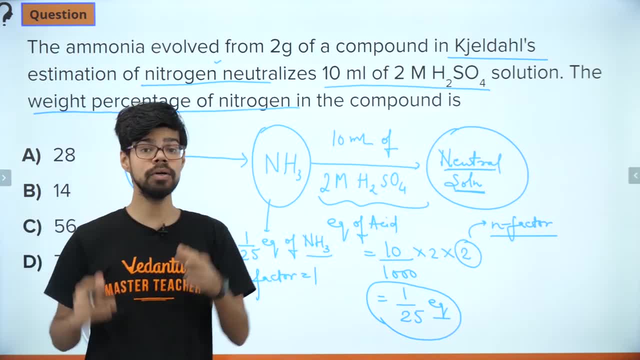 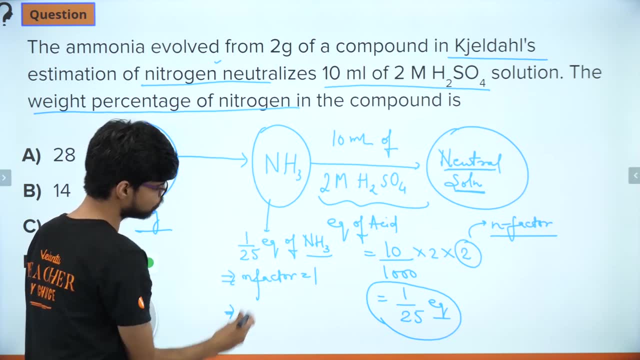 proton only to form NH4 plus. so because one molecule of ammonia only accepts one proton, so the n factor is one. so from here I can directly say: the moles of ammonia is 1 by 25 which is produced. so this is one part of the problem. okay, I. 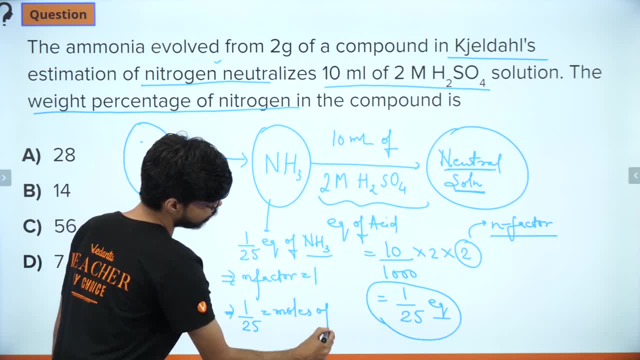 just got this, the scale out. okay. so to knowmouth is equal or equal to one by 25, it will give minus nN, which is what we can take out, and we'll pick up again. we sat well, we carried on. we have got present in our predicted problems in detail right now. 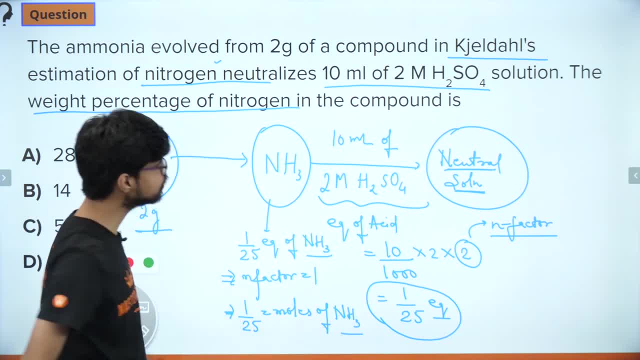 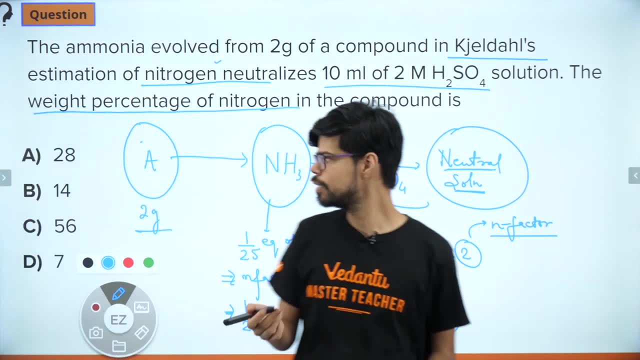 which we can take out if we sleepy. so we'll construct these on the second part to So. this is a simple titration from ammonia and H2SO4 and it is used to calculate the moles of ammonia. Now from here we can say: the amount of nitrogen here will be the same- all the nitrogen has. 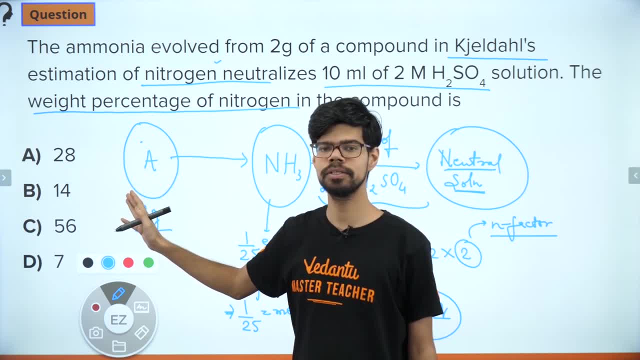 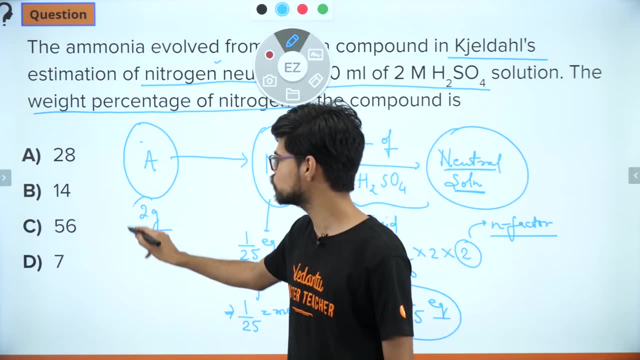 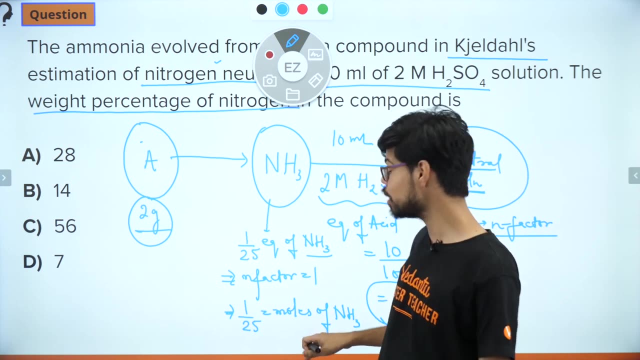 come from A. So now what is the second part of the problem? we have to calculate the percentage of nitrogen, So we know the total mass of the compound. We can also calculate the mass of nitrogen. We know the moles of ammonia. moles of ammonia will be equal to moles of nitrogen. 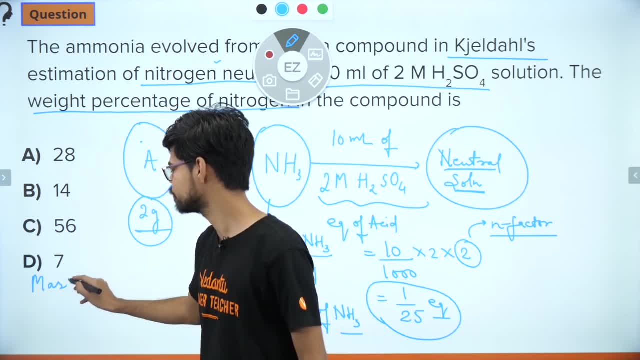 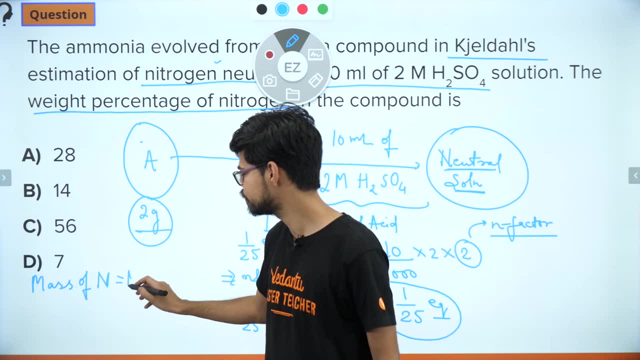 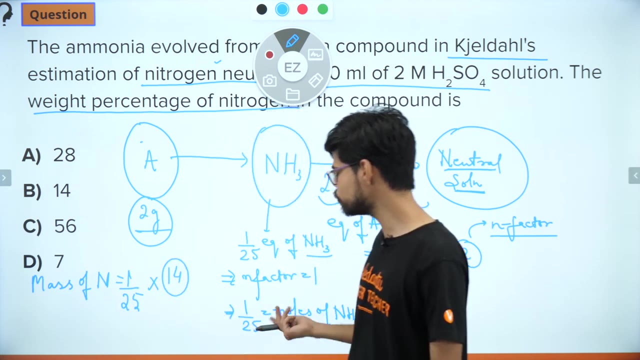 So mass of nitrogen will be moles, which is 1 by 25 into 14.. Now this is a critical thing. you do not have to write the mass of ammonia, you have to write the mass of nitrogen, Right, Because nitrogen is the element which is present here. 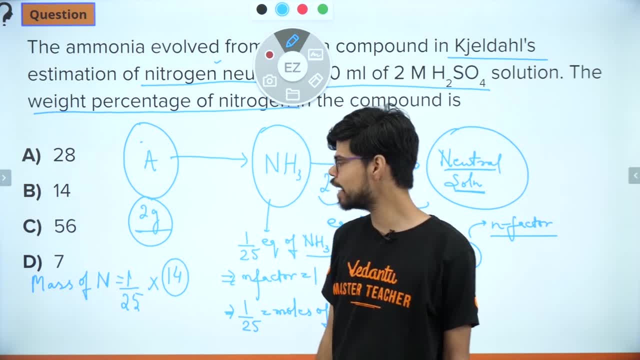 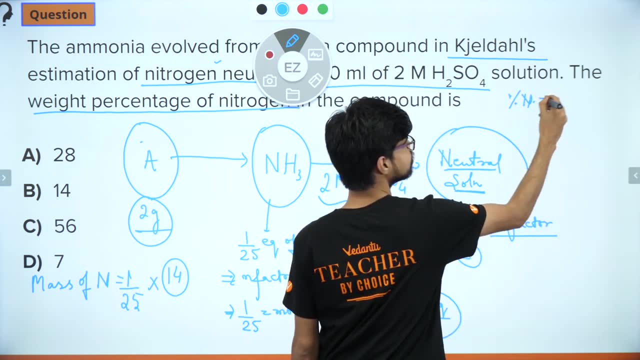 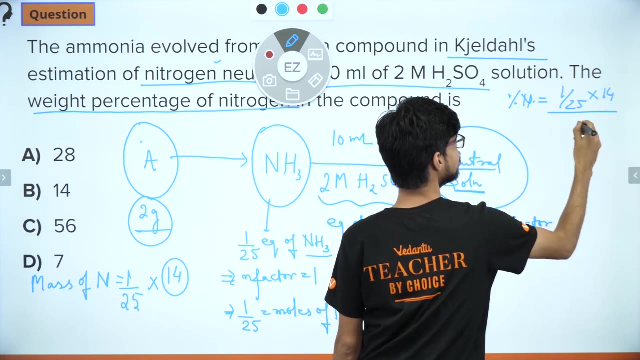 So this will be the mass of nitrogen. I hope you can calculate the percentage now. So percentage will be. let me do it here. So percentage of nitrogen will be mass of nitrogen, 1 by 25 into 14 upon total mass, which. 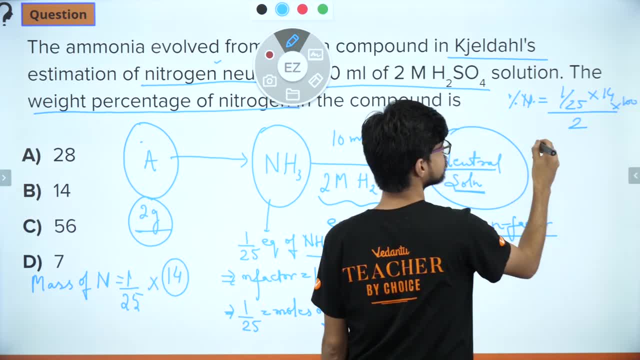 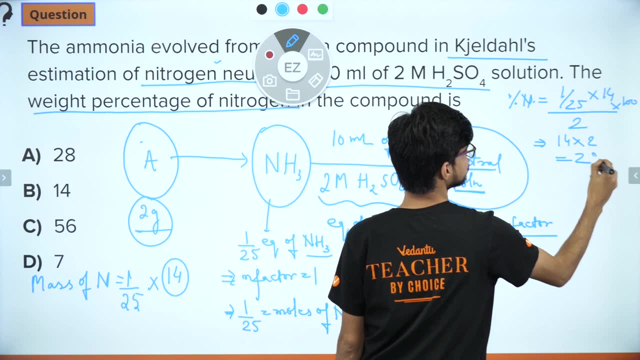 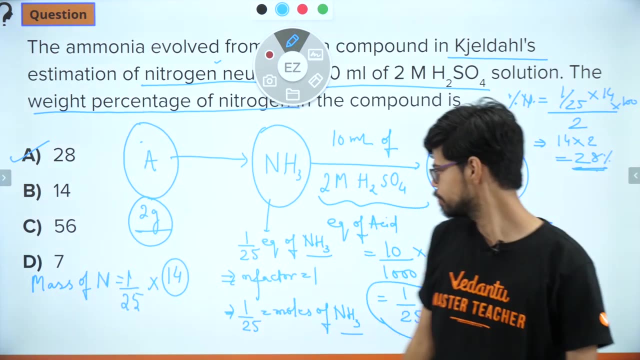 is 2 into 100. So it comes out to be 14 into 2.. 28 percent. Is it there? Yeah, we got it. Ok, Go through the solution once. let me summarize it. The Gel-Dahls method basically works like this. You heat the compound with something, something we do not really care. All the nitrogen here is converted to ammonia. we measure the amount of ammonia by reacting with H2SO4. We have, we know the amount of H2SO4, we calculate the moles of ammonia. form the moles of ammonia. 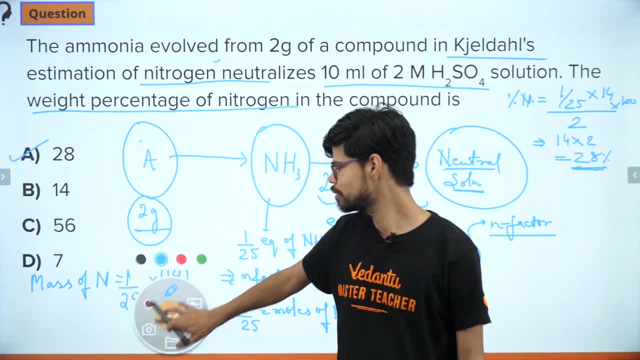 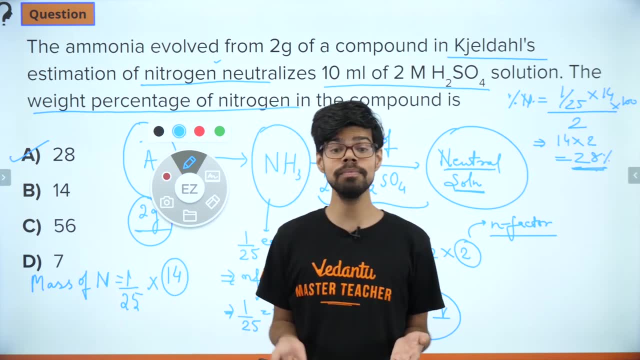 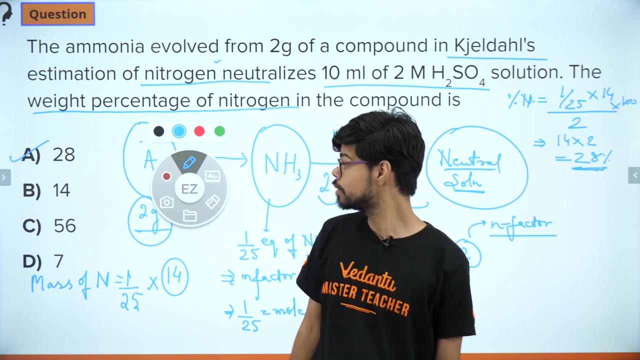 This is a Stevens' equation. we can get the mass of nitrogen right and from mass of nitrogen we can then calculate the percentage. this is a very standard problem and it is helpful in all the major exams. it is a practical method to calculate amount of nitrogen in any compound. okay, we are done with this. let's. 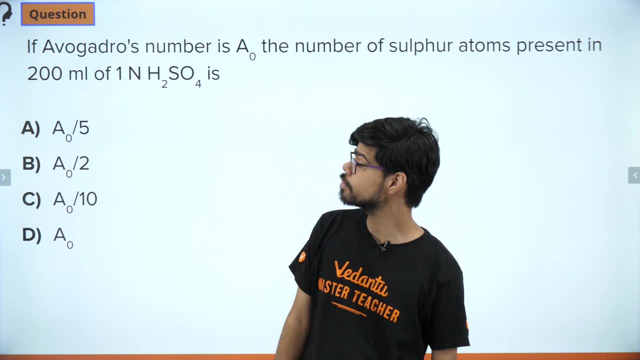 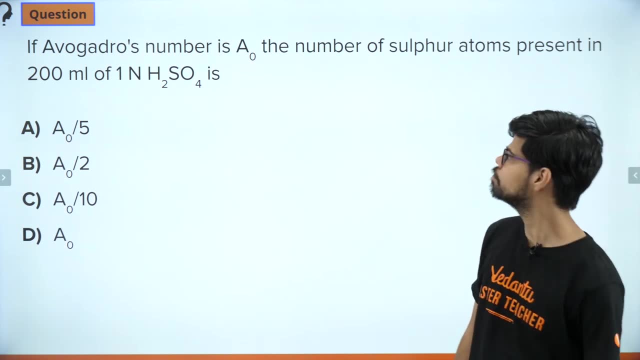 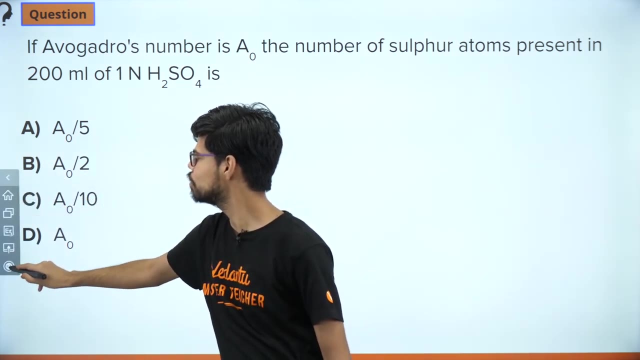 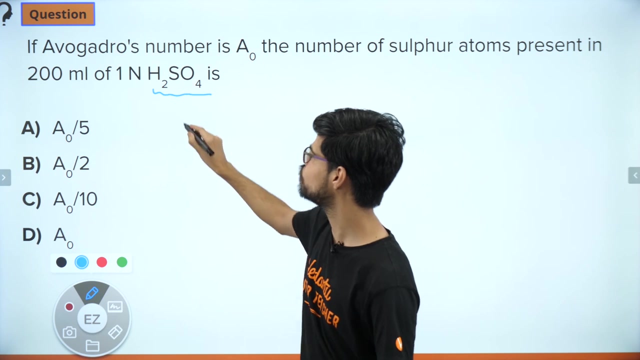 go to the next one. so answer is 28. this is a pretty easy one. i would like you guys to try it out. do it quickly, okay. so what does it say? number of sulfur atoms in 200 ml of some some h2so4? okay, let's do it quickly. we have to calculate the moles of h2so4. 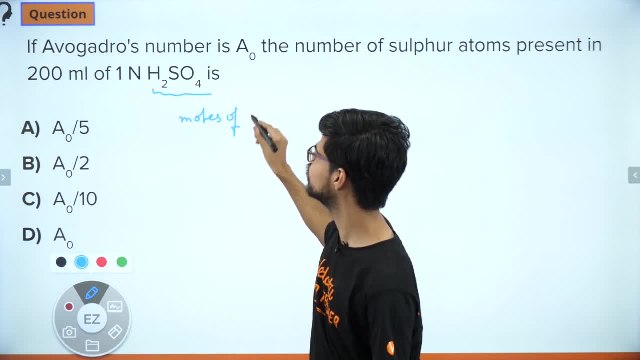 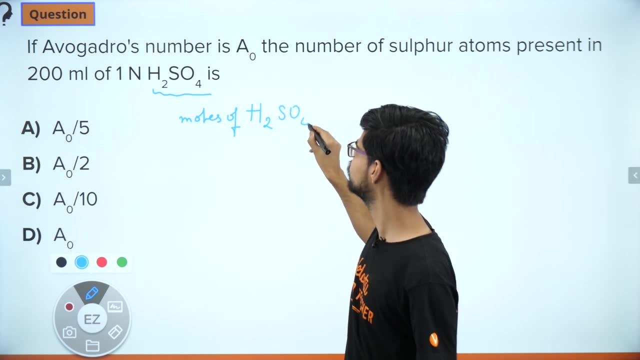 as we know, the every one h2so4 has one sulfur, so that will be equal. so moles of h2so4, and the only thing here is that we have to calculate the moles of h2so4 and we have to calculate the moles of h2so4. 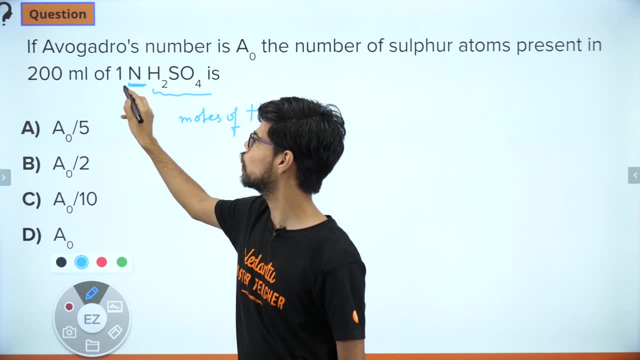 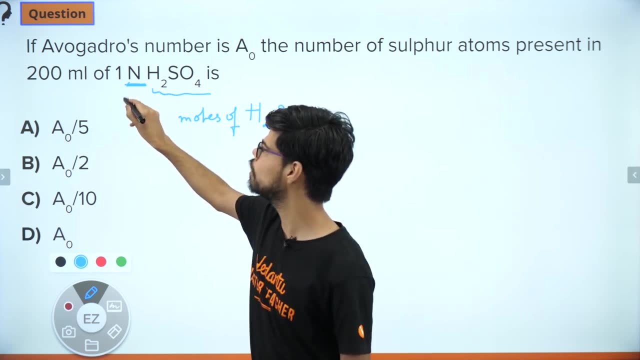 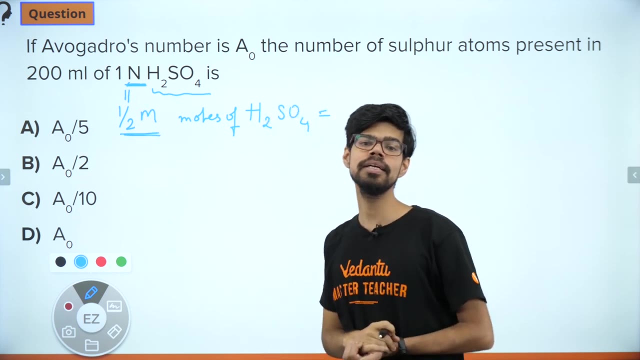 which can catch you out is: this is normality, not molarity. okay, so for h2so4 n factor is two, so one normal will mean half molar. this is the main thing, this is the only thing which can catch you out. so one normal means half molar because n factor is two, so moles of h2so4 will. 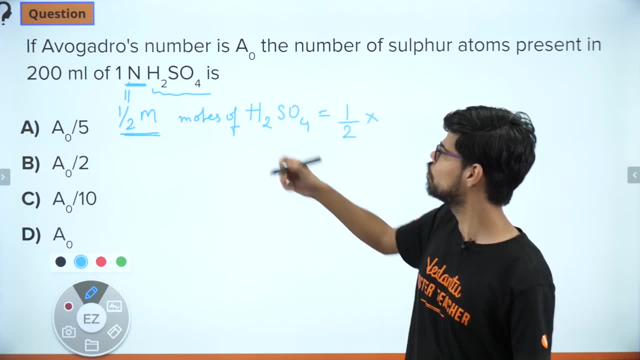 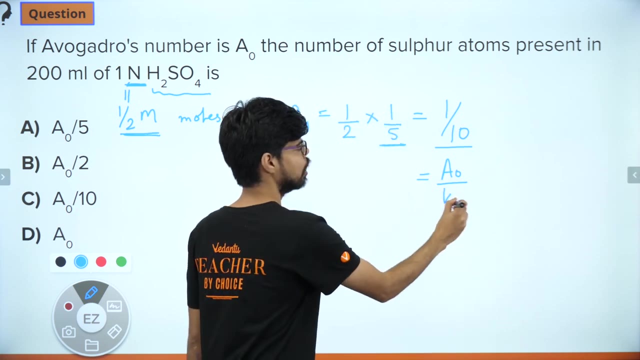 be molarity into volume. volume is one by five liter again. the second thing is that we have to calculate moles of h2so4, a one by five, by 10, and so on weeks. this is a foi Mechanism. nothing always rightότε are more liters a four unit will get. most of this is one by 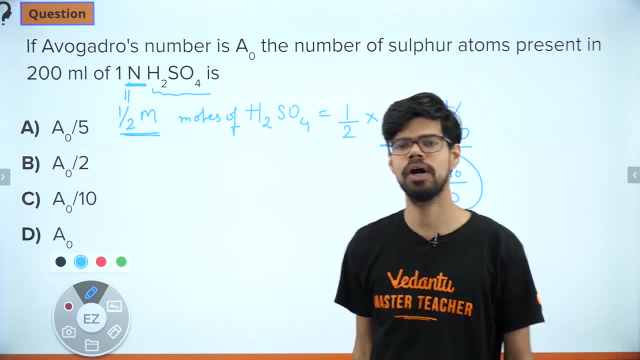 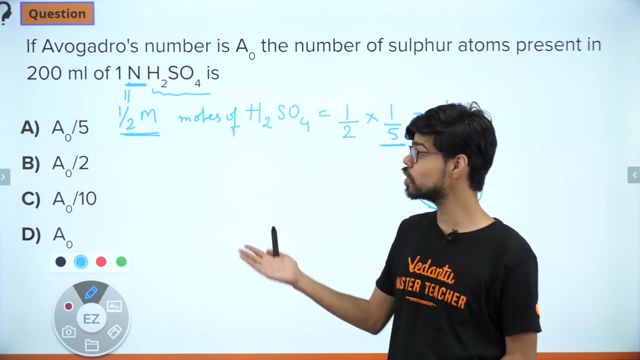 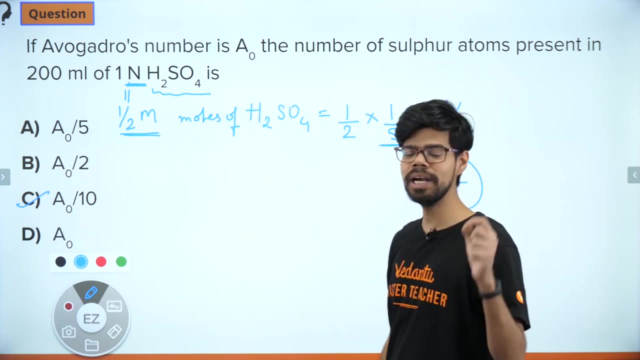 ten most. so basically a note by ten molecules. so out of sulfur will also be okay. i not by ten. very simple, and this is a question which i also appeared in an exam, so not all questions are a figure. if you can solve this, you can surely do anything. answer is C: the 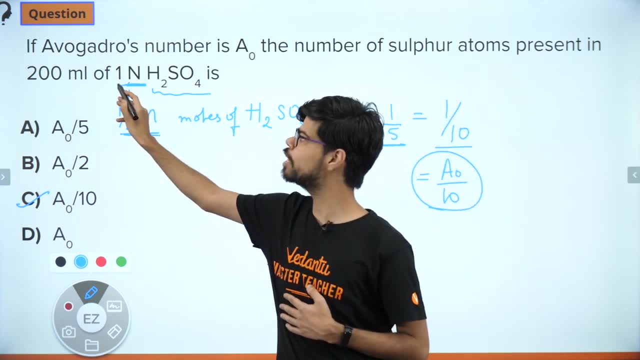 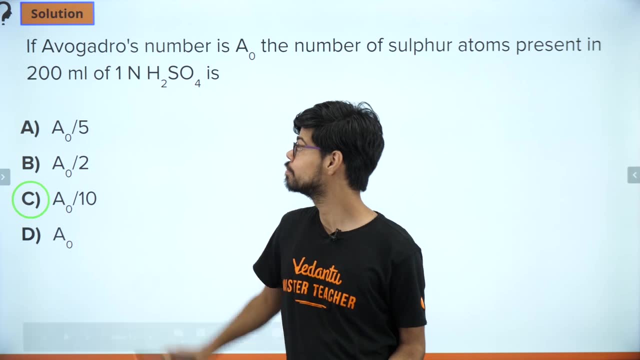 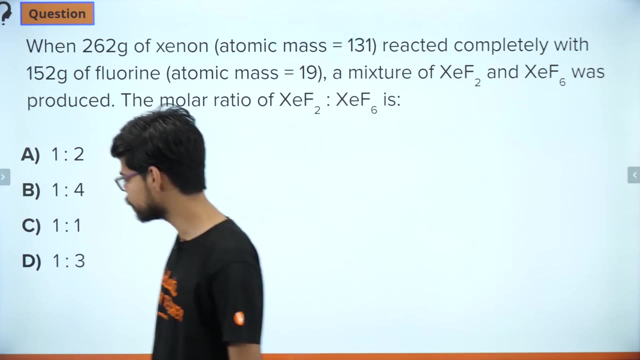 out in such questions is: don't make mistakes. read the question carefully. don't be hasty. hastiness will cost you marks. okay, that is what this question teaches you. so answer is c. oh my god, next one. okay, now, this is an interesting question. please go through it. you can try it. it will take. 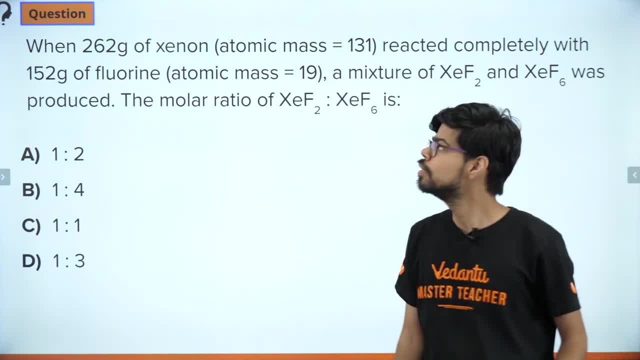 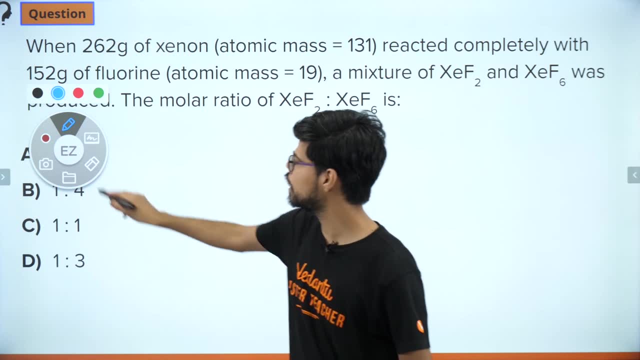 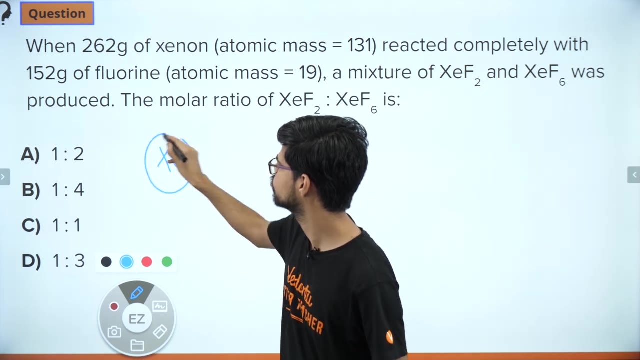 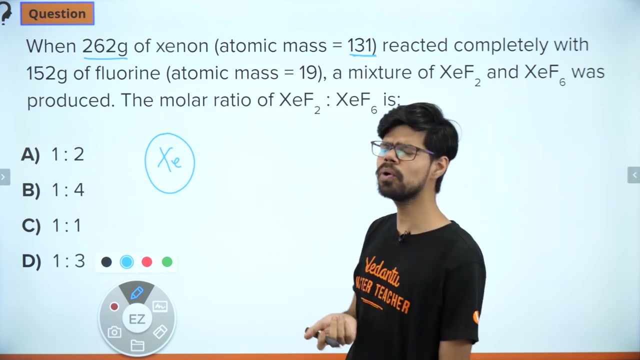 some time. okay, let's work it out. so what does the question say? so we have zenon. so what does it say? we have some xenon and the mass of xenon is given along with the atomic mass. so first thing you have to do always in such questions is convert to moles. we cannot do. 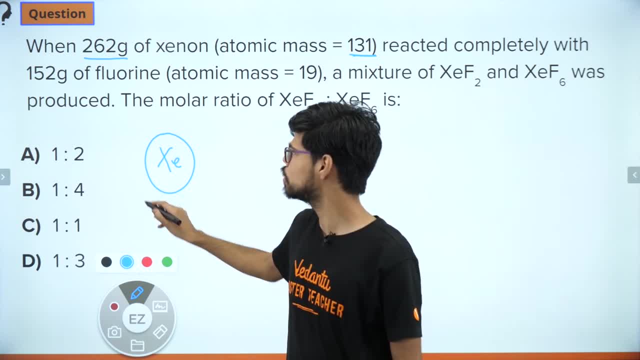 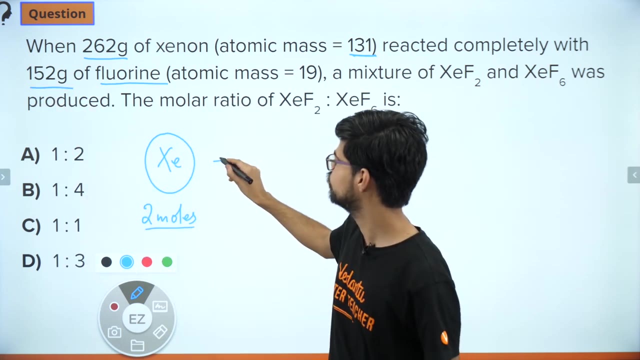 anything with mass convert to moles. so, as you can directly say, 262 by 131, it's two moles. so we have two moles of xenon, xenon gas. it is monoatomic and we have some flow in and the mass is 152. okay, so we have some fluorine gas, f2. 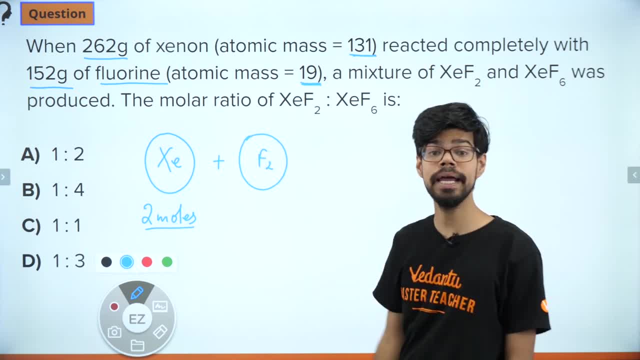 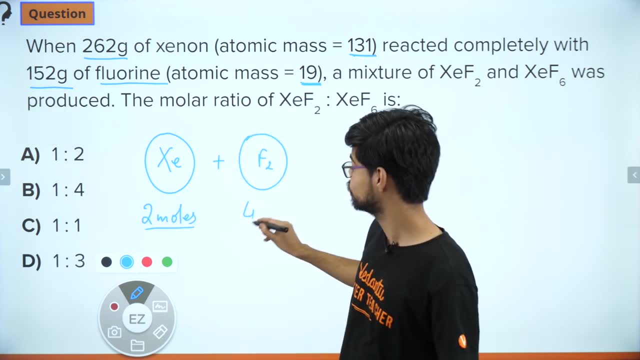 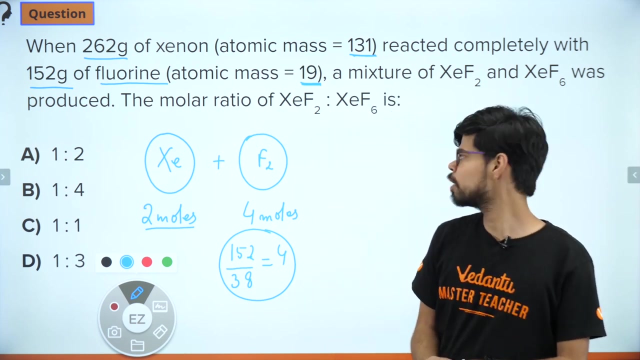 atomic mass is 19, molecular mass is 38 and i guess you can identify this number. it is a multiple. you will get four moles, so 152 by 38 should be four, i guess. check it out, okay. okay, so we have some amount of fluorine and some amount of fluorine. 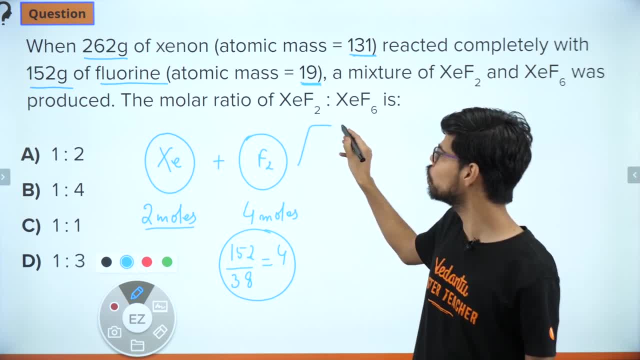 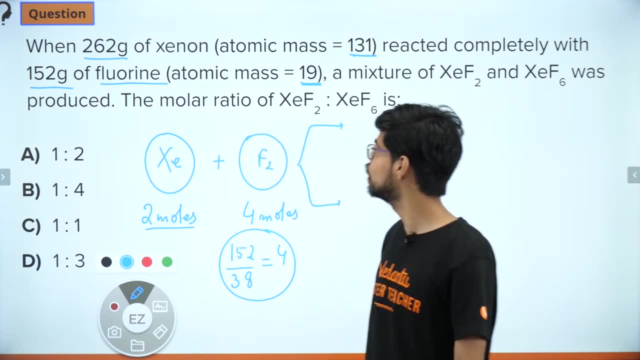 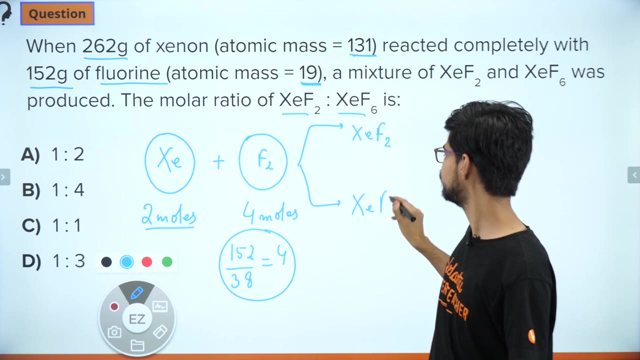 now the tricky thing is when they react they form two compounds according to the question. in reality they do two, more than two, but in the question we have to deal with two compounds, and they are xcf2 and xcf6. so we have some xcf2 and we have some xcf6. okay, now the question is: 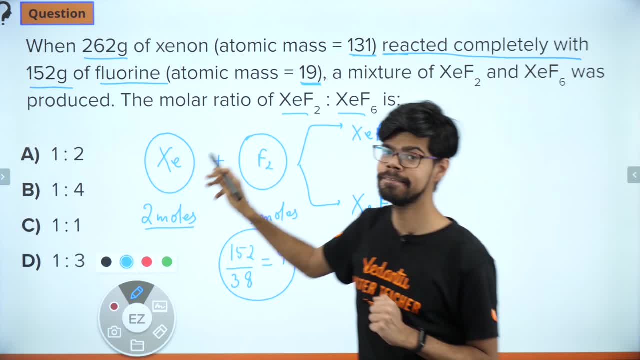 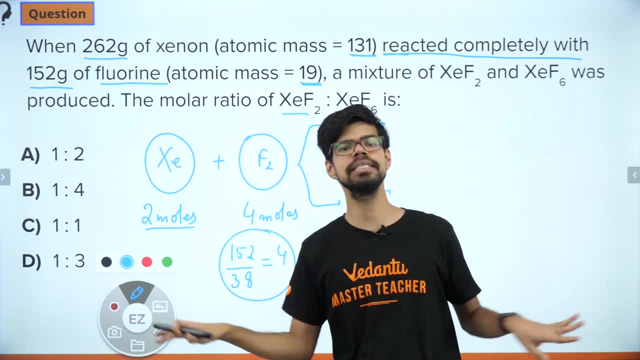 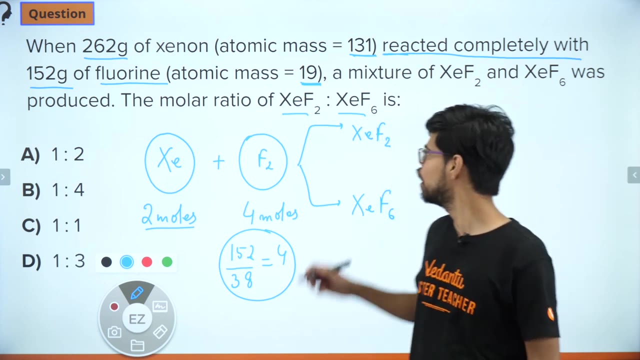 if all is reacted completely, it means, when they react, all of xenon and all of fluorine has been consumed. nothing is left. this is the main point. nothing is left, and using that information, we have to calculate how much of this and how much of this is produced. okay, so this is the question. 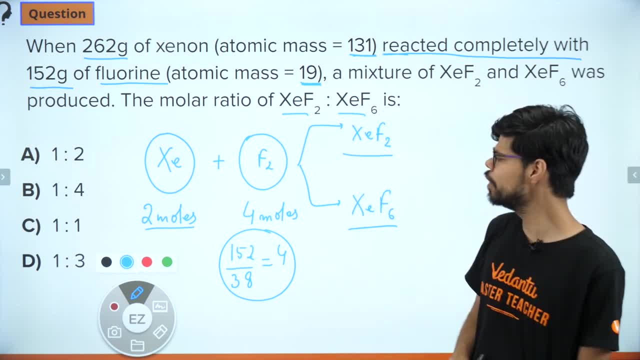 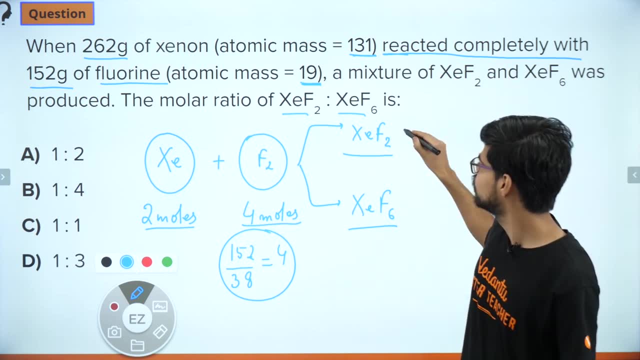 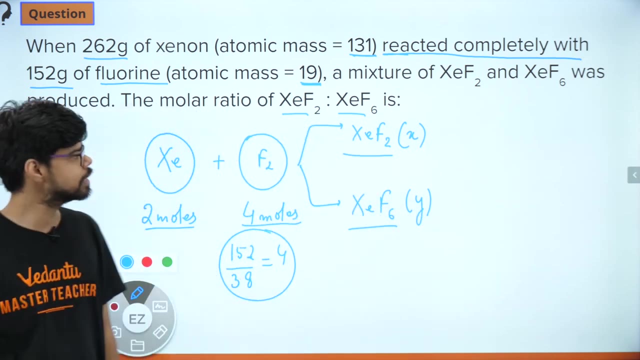 it might appear a little tricky, it's pretty simple. so what we can do is we know the moles and we have to calculate the amount of xcf2 and xcf6. let's say this is x and this is y. okay, i have assumed x- amount of xcf2 and x of y amount of xcf6 is produced. okay, so now we will form two equations. 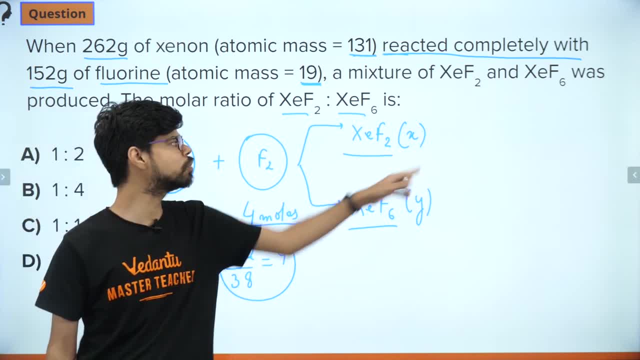 and we will just solve them. so for producing x moles of xcf2, x moles of xc will be fused and to produce y moles of xcf6, obviously xcf2 will be fused and to produce y moles of xcf6, obviously. 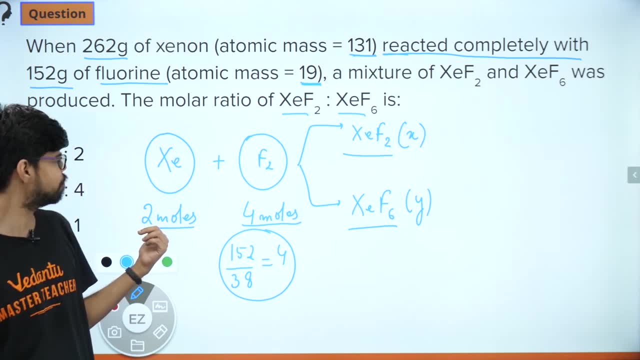 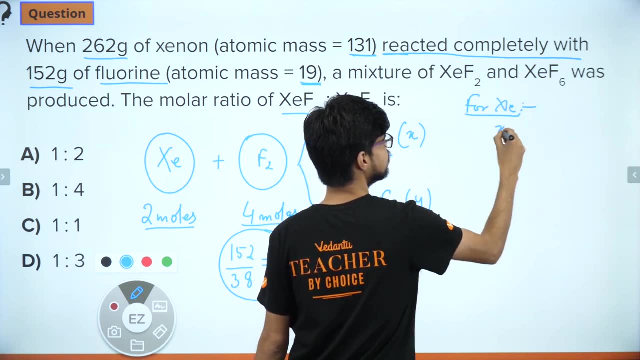 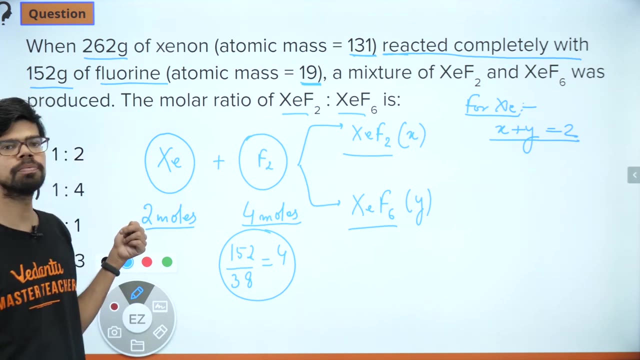 one y moles of xcf, xc will be used. so i can directly write for xc or xenon, x plus y will be two straight forward right. each of these use one mole of xcf6 to produce xc2 produced. so amount of x plus y must be two. okay, you can do it directly as well. you can write x. 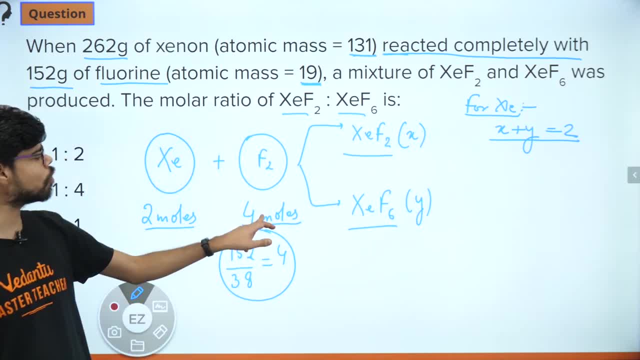 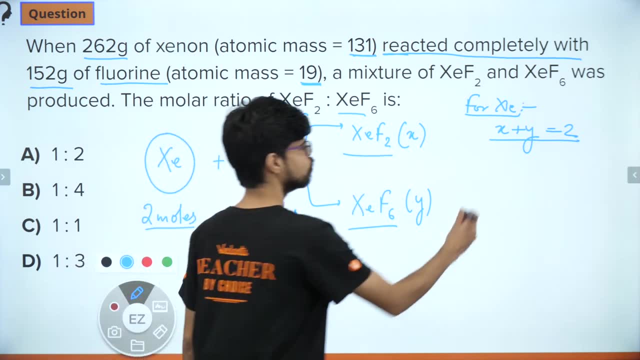 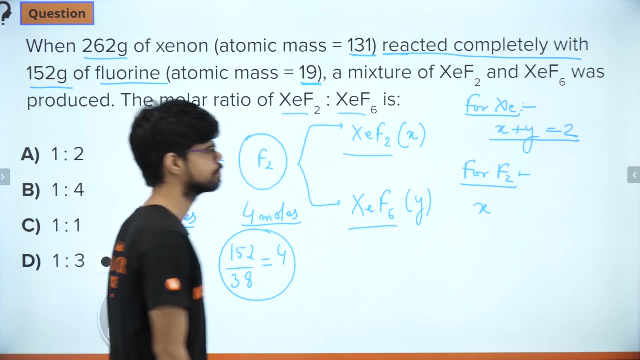 and two minus x, and that is fine as well. now the main thing is four moles of fe2, f2 we have. so for one mole of this, one mole of f2 is required, right? so what can i write for it? fluorine x, and for one mole of this how many fluorine are required? you have f6 here. 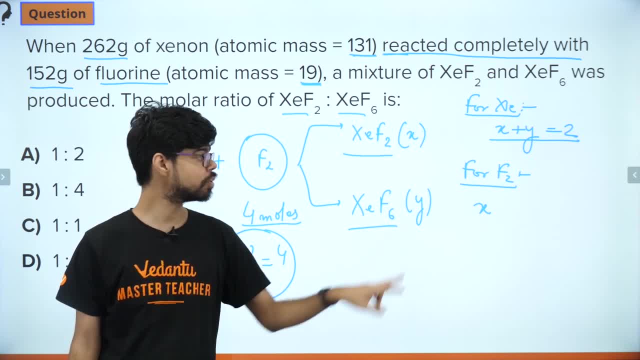 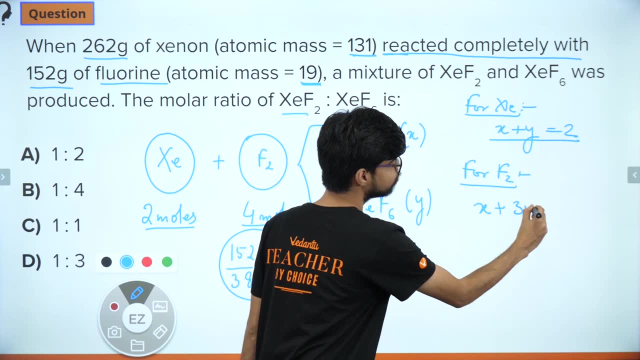 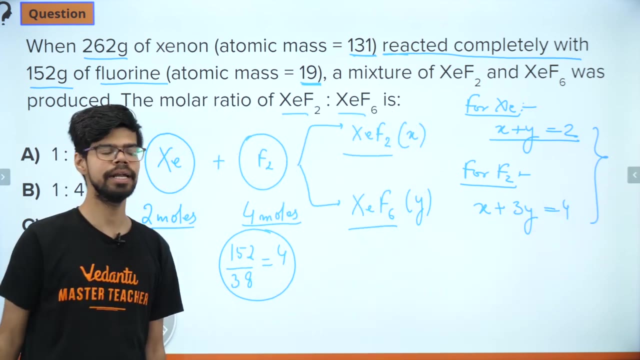 so i can directly see it will require three moles of fluorine. so for one y you require three moles of fluorine. so amount of moles of fluorine will be three y for xcf6 and the total is four. we get these two equations. i think you can directly solve it. when you solve it. 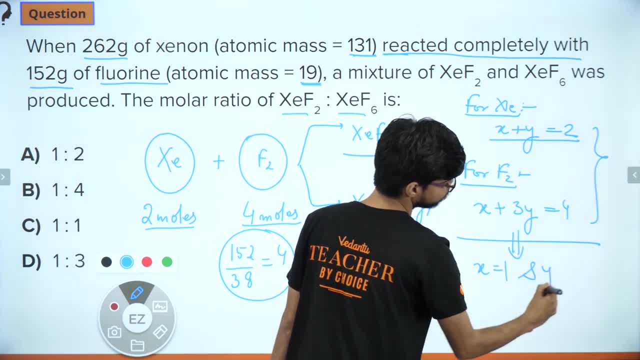 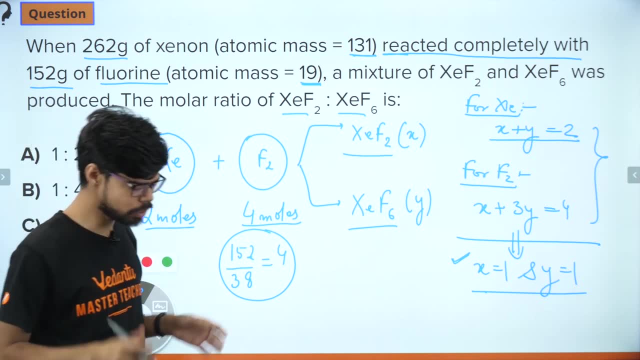 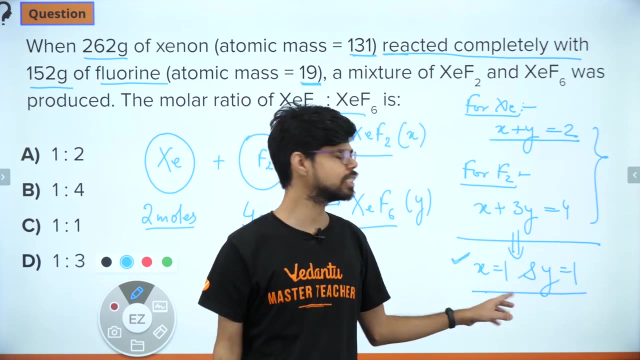 you will get x equals to one and y equals to one. so it is pretty simple when you solve it in moles. so again, the simple thing is always convert mass to moles and f required and most to mass. here we don't know or what. we don't need it because x is one, y is one. we are only asked the ratio. 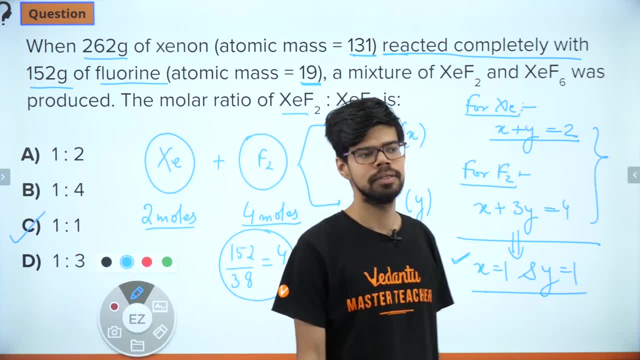 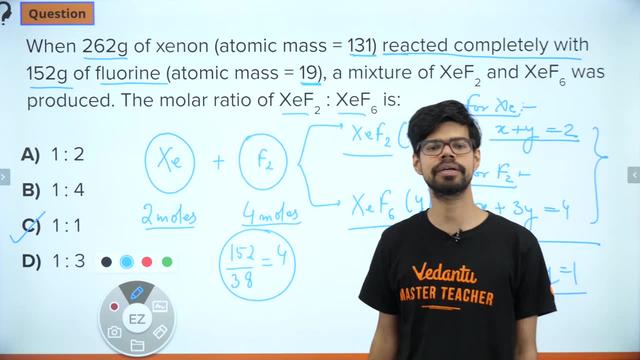 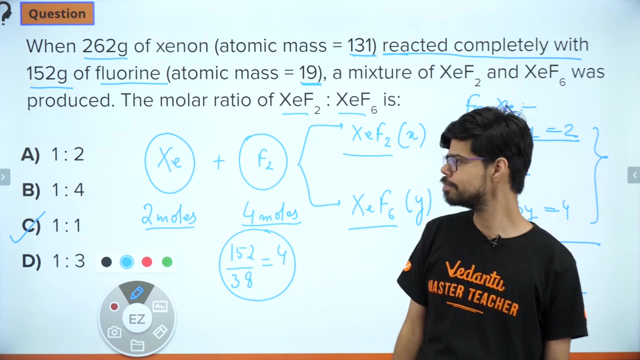 the ratio will be: c: one is two one. so this is another type of question, basically when two reactants react to produce more than one product. okay, so given some constraints, we can calculate such questions. okay, this is another variety. it's done. check out the answer, let's see. 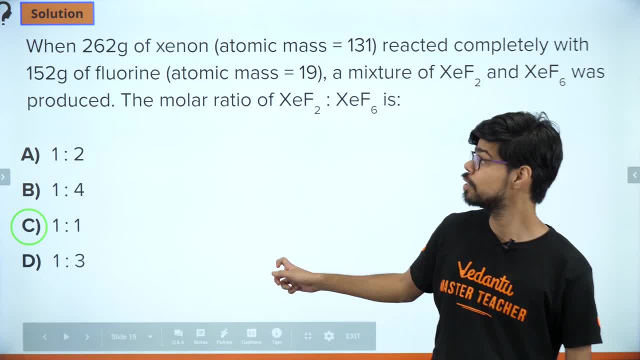 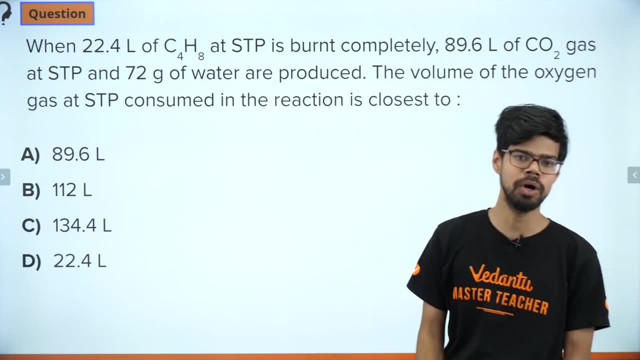 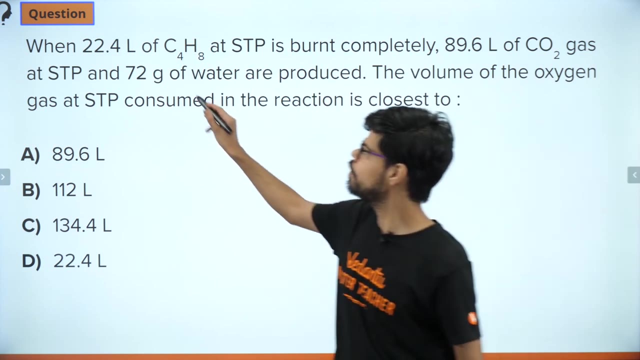 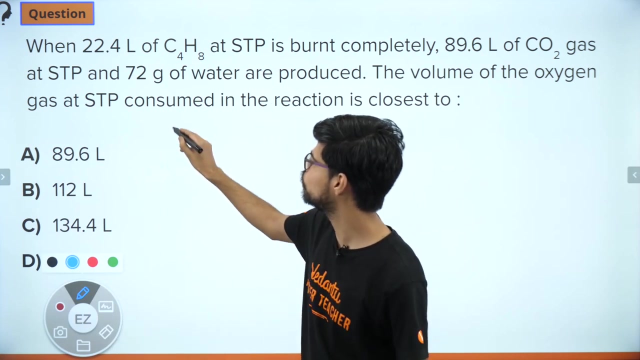 okay, this is another question from previous years. let's go to the next one. okay, this is in gases. now go through it. try it. pause the video. okay, let's do this again. i'll draw diagram. we have some gas which is a hydrocarbon and the hydrocarbon is C4H8, so we have C4H8. 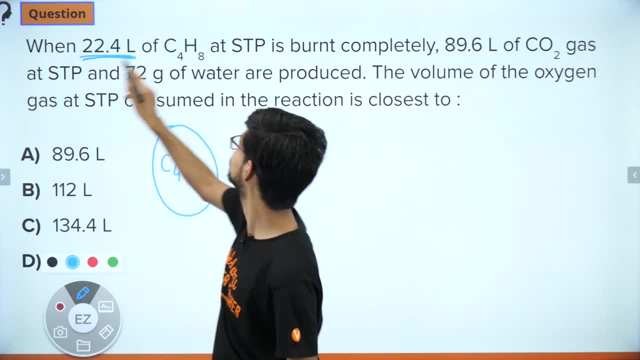 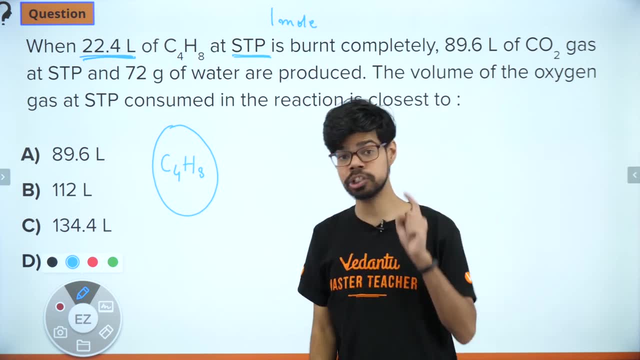 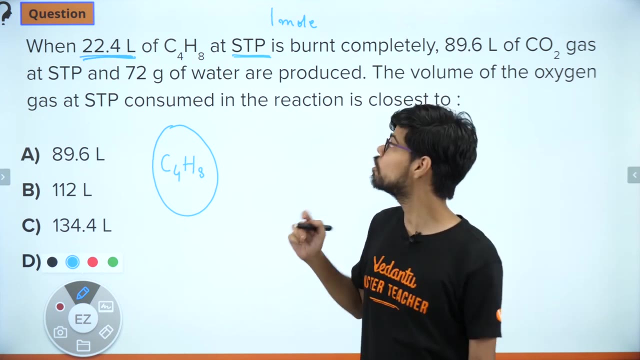 and we know the volume of it and what is the significance of number and it is written STP. we know one mole tablespoon. so basically, whenever we are given volume for a gas- and this is also only for a gas- many people in class, especially in class 11, get confused with volume. this only works for gases and 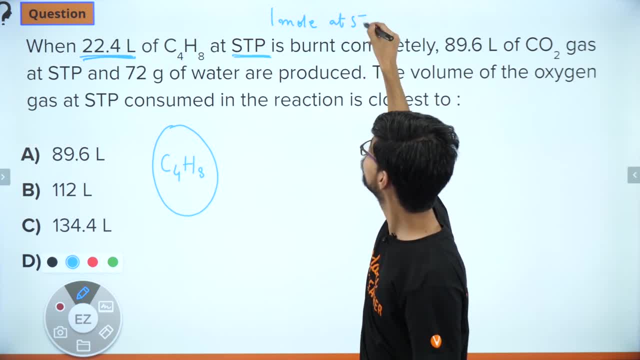 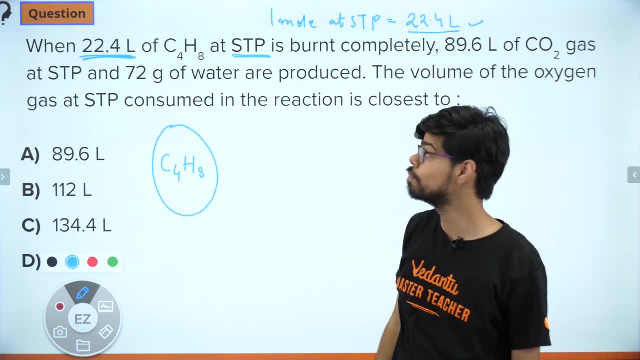 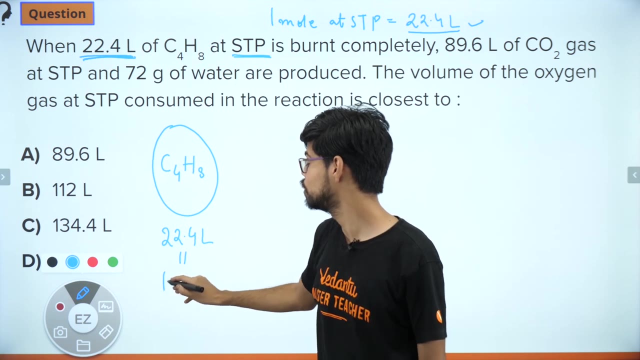 what is the result? one mole of a gas at stp- whatever the gas is, it doesn't matter, for any gas is 22.4 liter. this is the result which we use. this is called avogadro's law. so 22.4 liter- again, liters don't really matter, we will just convert it to moles. so it is one. 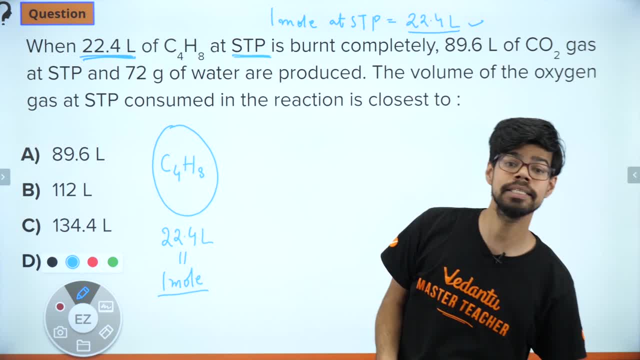 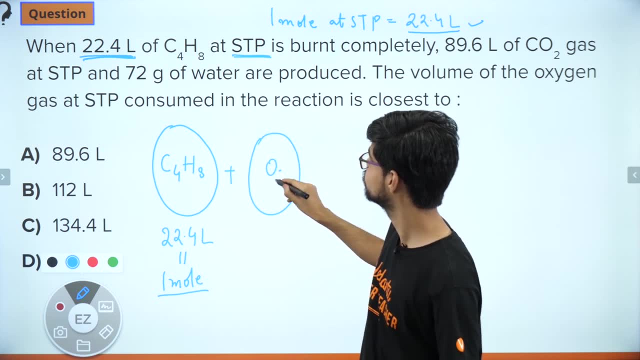 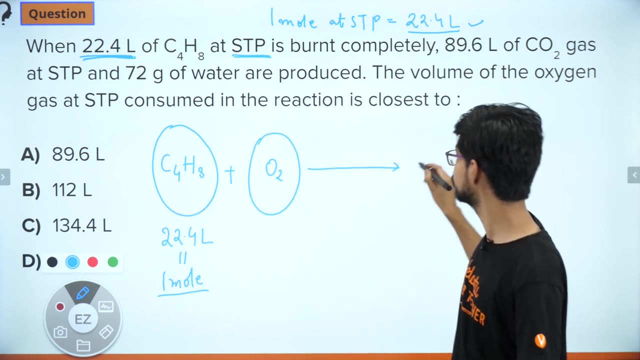 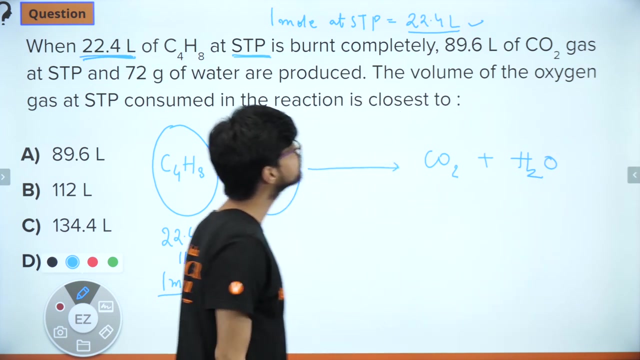 more. so this is another way of basically saying: one mole of a gas: okay, it reacts with oxygen. when we say burn, it is reacting with oxygen. okay, what does it produce? it produces whenever hydrocarbons, when we know we produce co2 and we get water. so what does the question? 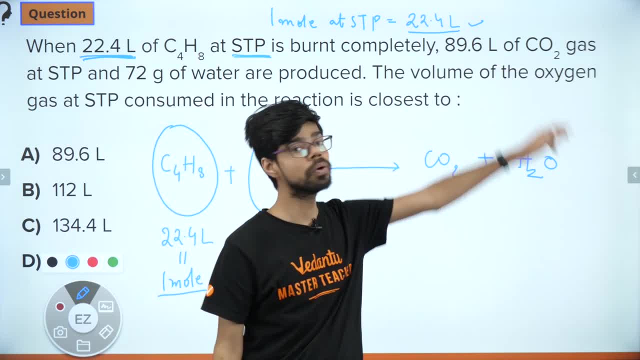 say 89.6 co2 gas? 89.6 means water. So this is what we get. So what does the question say 89.6 co2 gas? 89.6 means water. So what does the question say? 89.6 co2 gas? 89.6 means water. 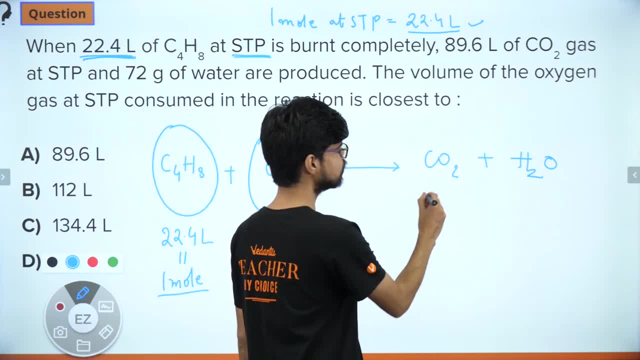 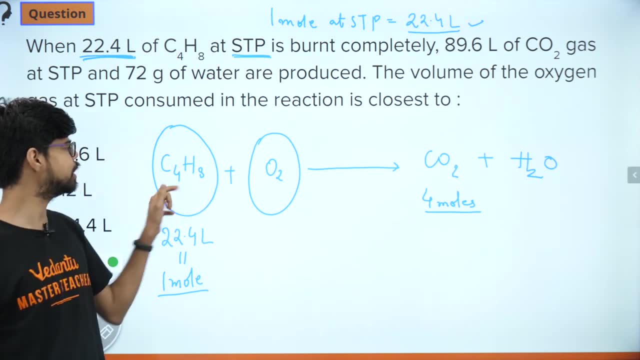 So this is what we get: 22 into 4.. So this is 4 moles. You can just divide it And obviously we know this already: 1 mole of C4H8, we have 4 carbon atoms, So obviously we should get 4 CO2 for 1 mole. 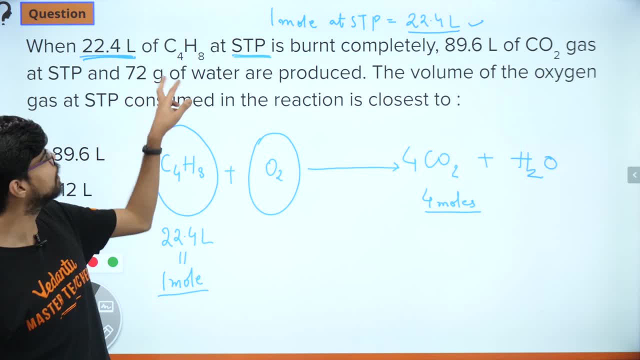 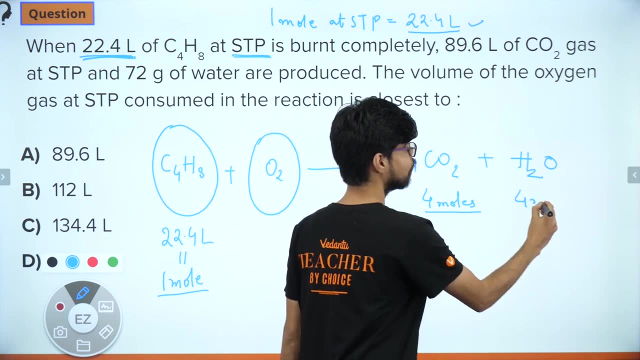 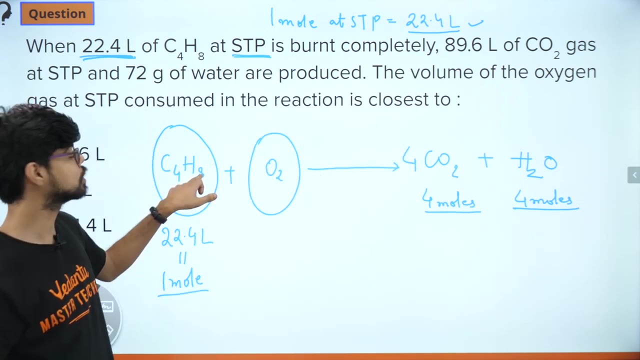 right. If we balance the equation, So that is obvious And we get 72 gram of water. 72 grams Molecular mass is 18.. So again 4 moles, And that is also something which you should already know. 1 mole has 8 hydrogen. 8 hydrogen will produce 4 moles of water, because 1 water 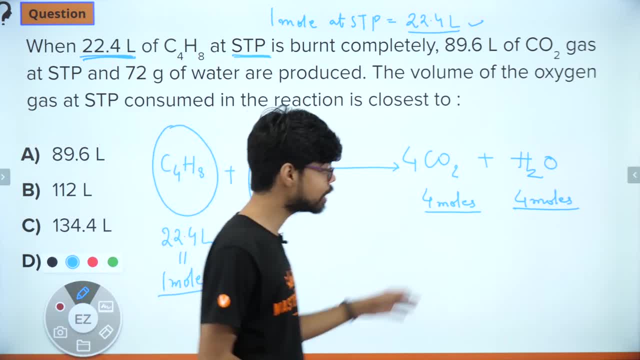 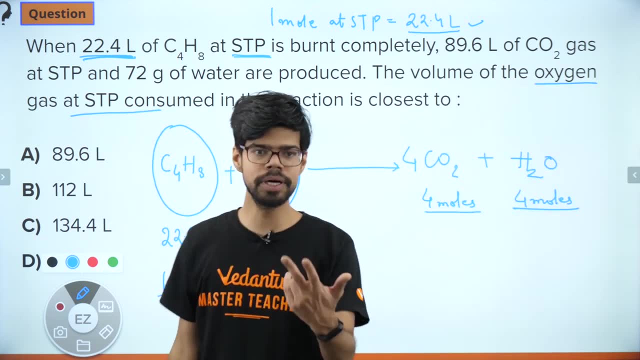 has 2 hydrogen. So this is the data which is given, not really required. We can directly calculate it. Now the question is: what is the amount of oxygen consumed? You can do it 2 ways. You can either balance the equation. 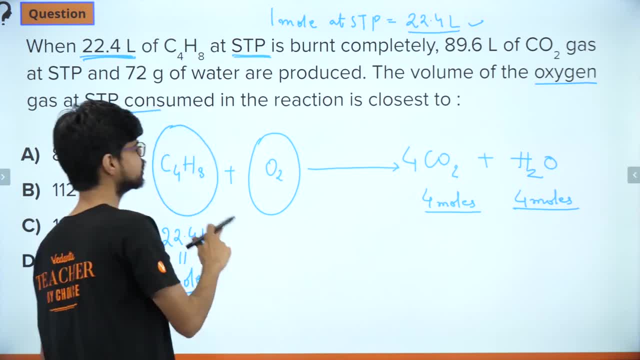 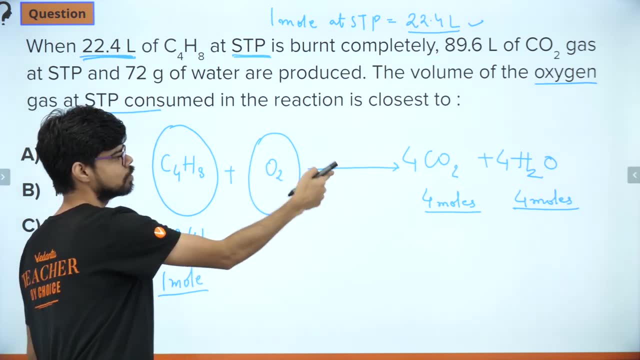 Which is the better way. If you balance the equation, you will get 1. C4H8 is 4 CO2 and 4 water, which we already know. And now count the oxygen, 8 plus 4.. So you will get 6.. 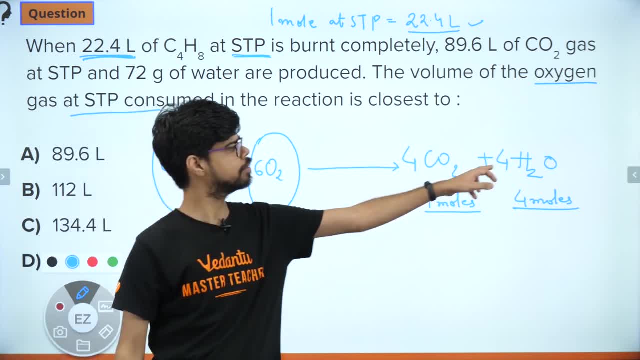 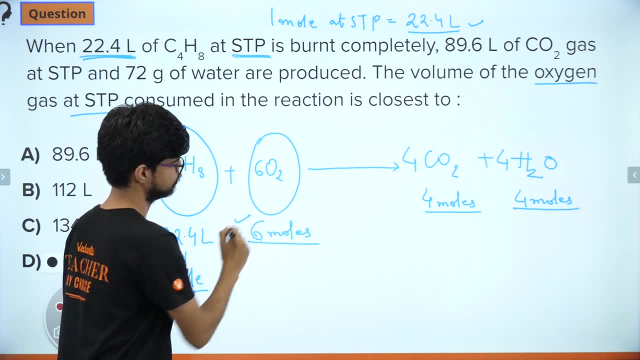 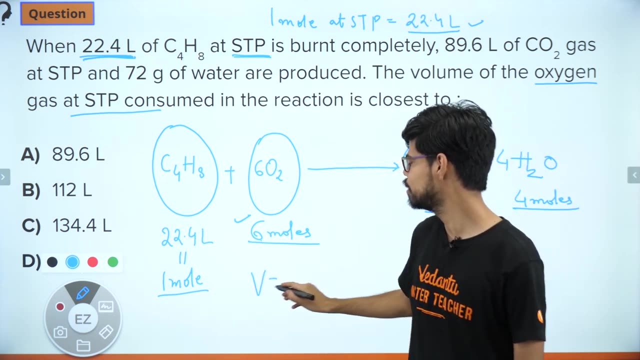 Right. Check it once: 4, 8,, 6 CO2.. So for 1 mole we will require 6 moles Right, 6 moles Right And 6 moles is So volume will be 6 into 22.4.. So how much it will be? 6 into 21,. 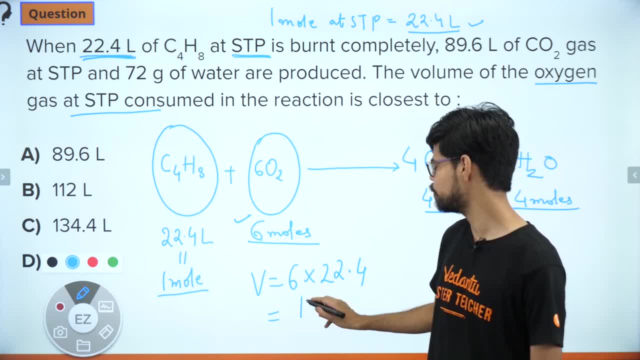 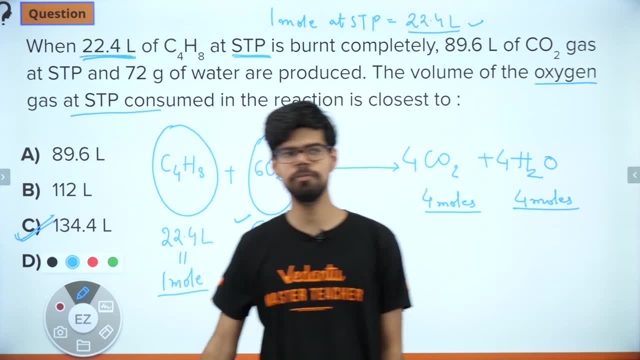 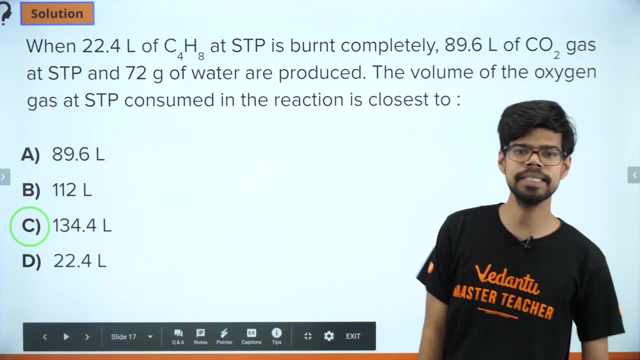 20,, 132,, 6,, 4, 134.4 liter. So pretty obvious. Just you have to do basic stoichiometry, convert it to volume, Volume to moles, moles to volume. Okay, So this is the answer. Let us go to. 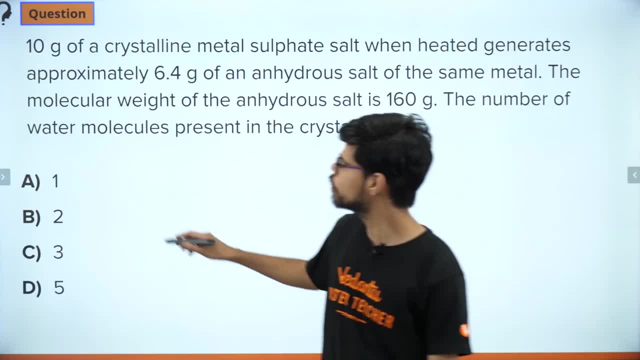 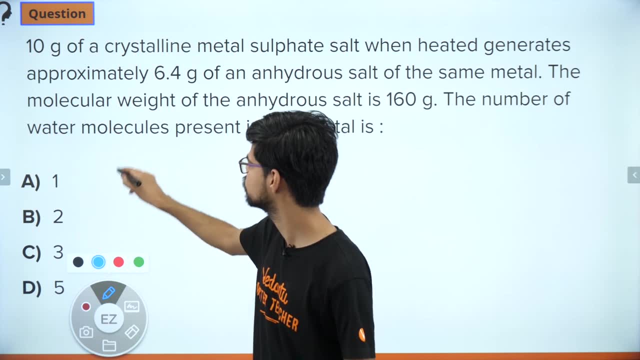 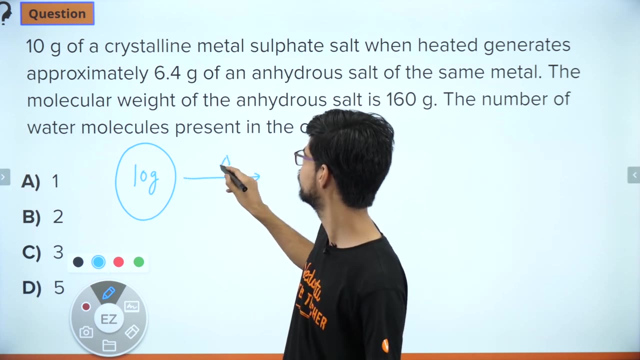 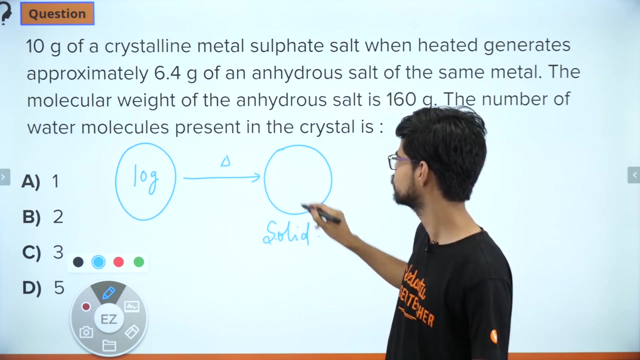 the next question. Okay, So we know in the equation we have 10 grams of a solid, 10 grams of a solid, and when it is heated you get a solid residue which doesn't have any water, and this is 6.4 grams and rest is water which. 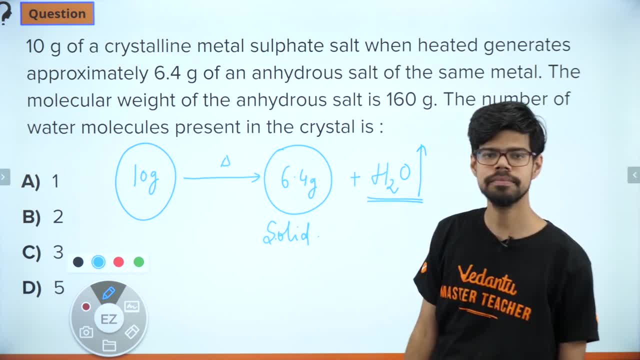 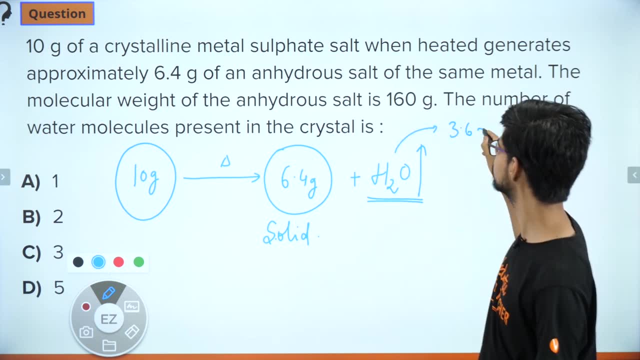 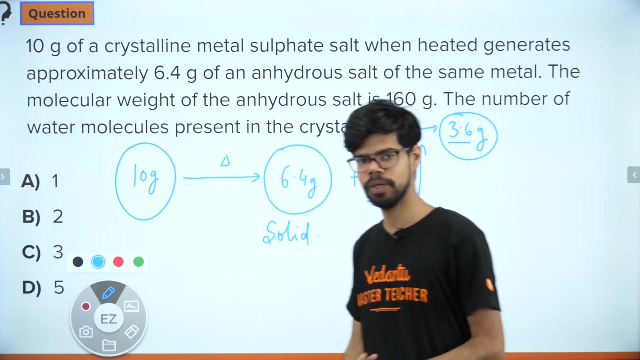 evaporates. okay, up from here we can simply say amount of water will be what. easily 3.6 grams, simply mass balance. this should be this plus this. so this is 3.6 grams. now we have to find the amount of water molecules in the crystal, okay. 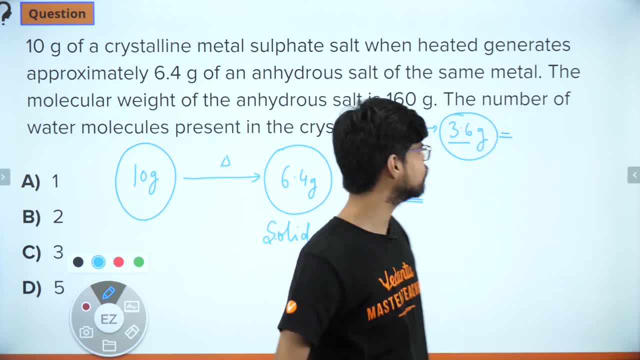 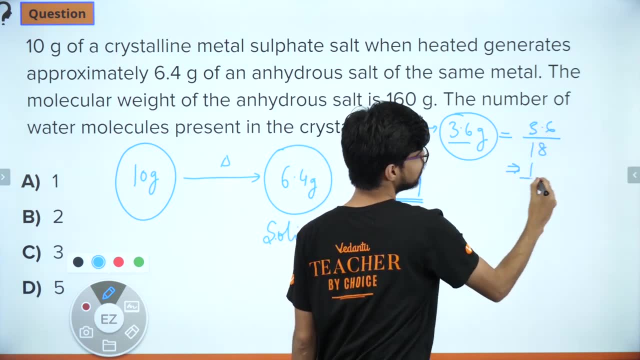 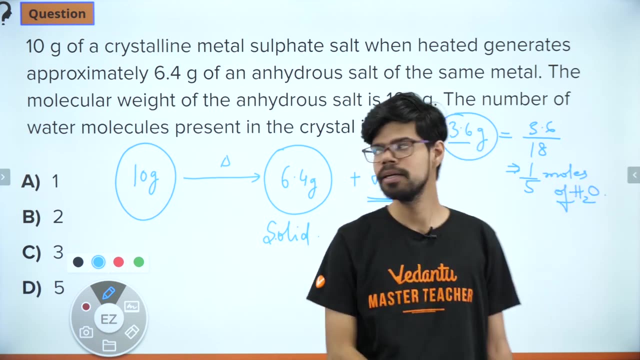 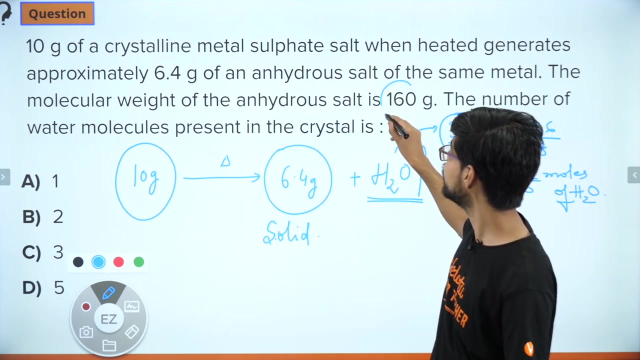 so we can see, from 3.6 grams you can convert it to moles, so it will be 3.6 upon 18 and this will be 1 by 5 moles of water. so this is the first part we get. 10 grams of the crystal produces 1 by 5 mole and the molecular weight of the 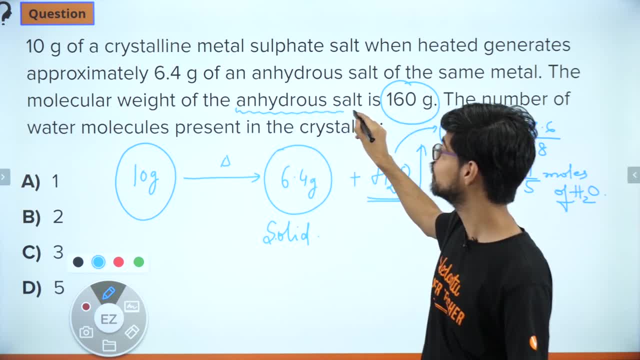 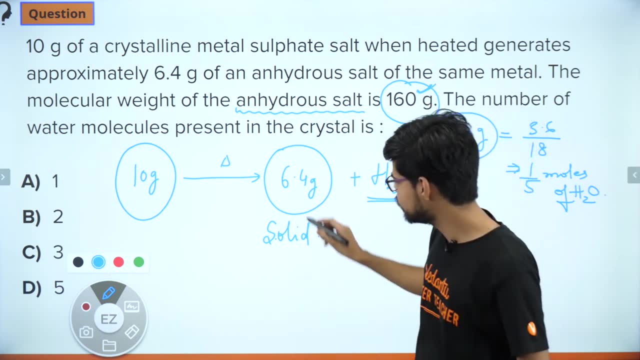 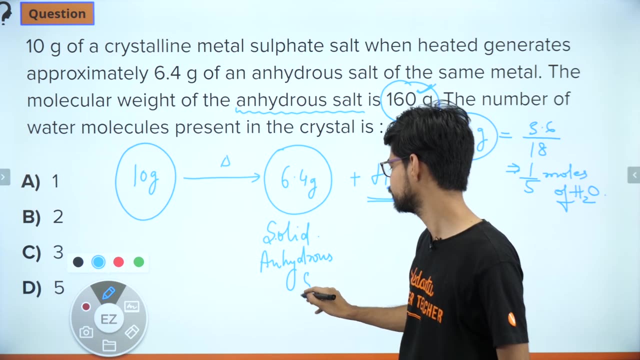 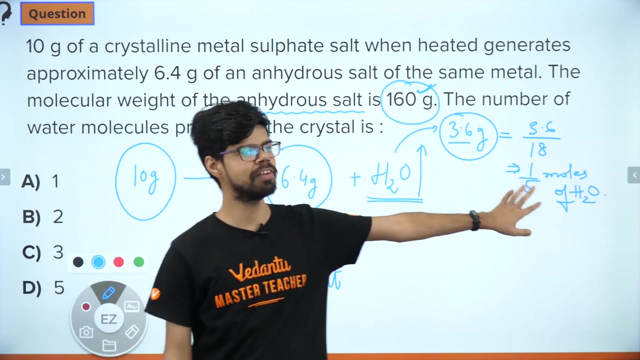 anhydrous salt. this is the important thing, and hydra salt with us, without water, is 160. okay, and this is our anhydrous salt. so now you can work out what to do so we can say, for 6.4 grams we have 1 by 5 moles, okay, don't. 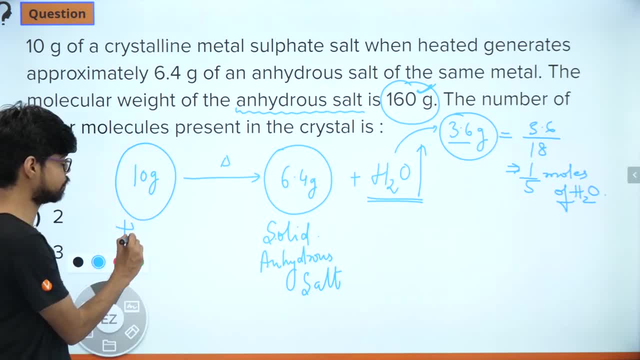 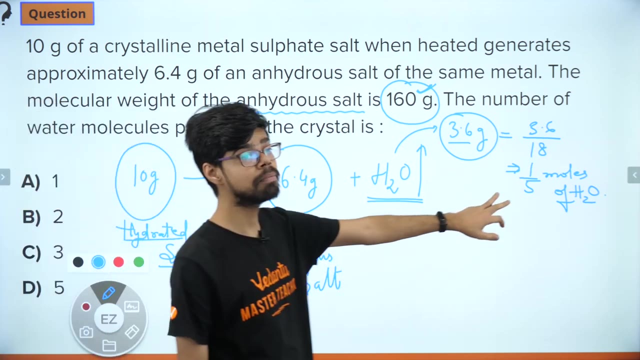 make a mistake of taking 10. this is the hydrated salt, so 6.4 grams combined for 4 moles and we'll get 60.. a litre of water for the בדunate of that is based on the tolerance delivered by Ecztasy anhydrous. 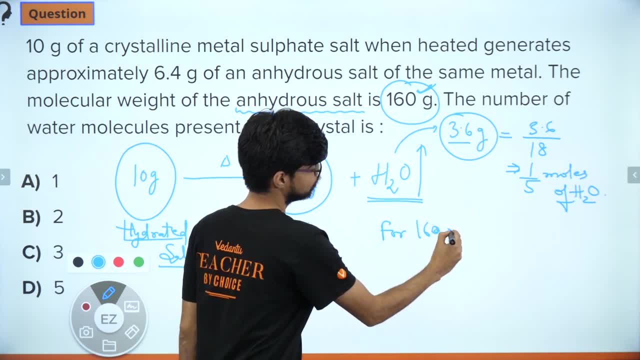 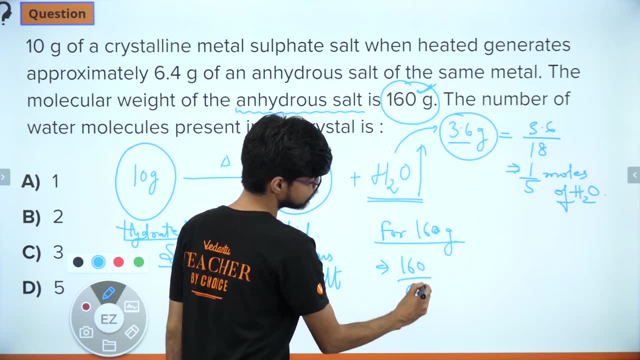 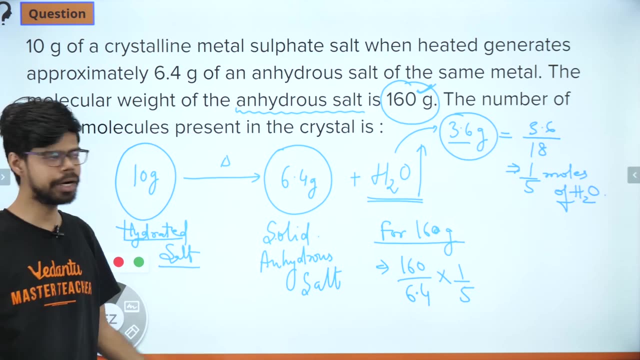 salt. so for 600 grams, so for 6.4 grams of the anhydrous salt, without what an address means without water. we have 1 by 5 moles of water, so we have to calculate 1 by 5. Can you understand why is this? for simple unitary method, if 6.4 have 1 by 5. 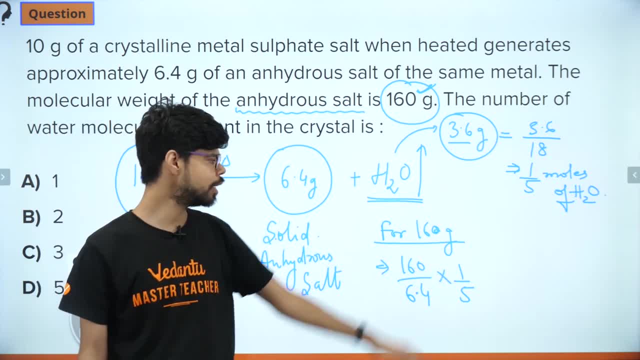 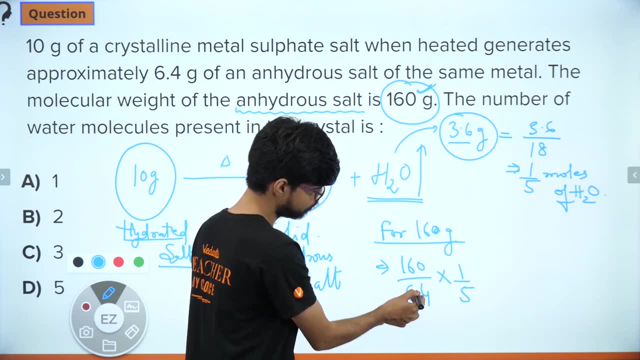 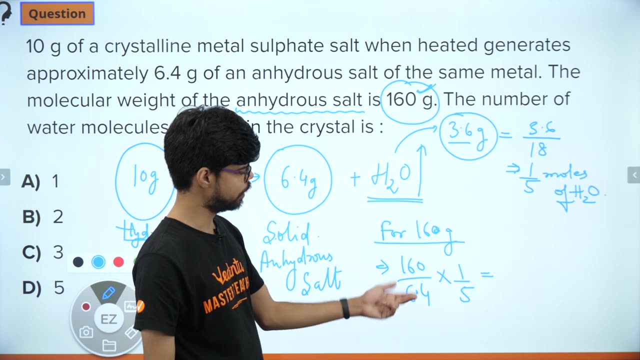 Then 160 grams will have 160 point upon 6.4 into 1 by 5.. So I guess this will be: This is 18 to 2, 6.4. Just calculate this 32. This into 5 is 32, 32, 5 size 160.. I guess yeah. 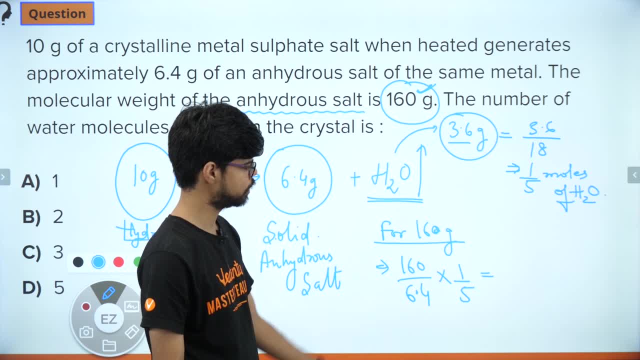 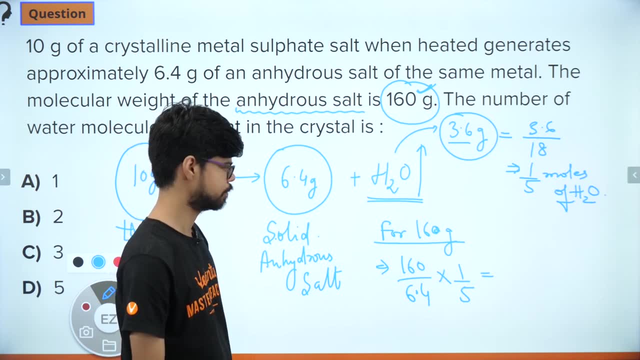 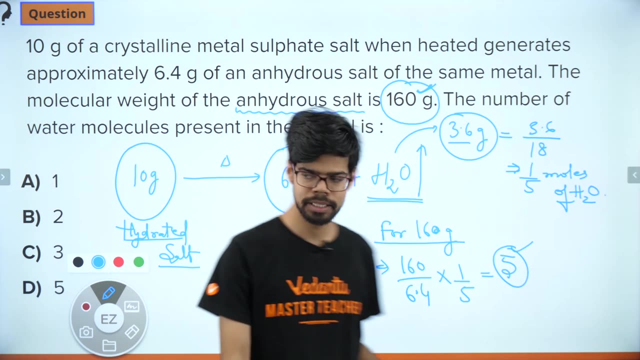 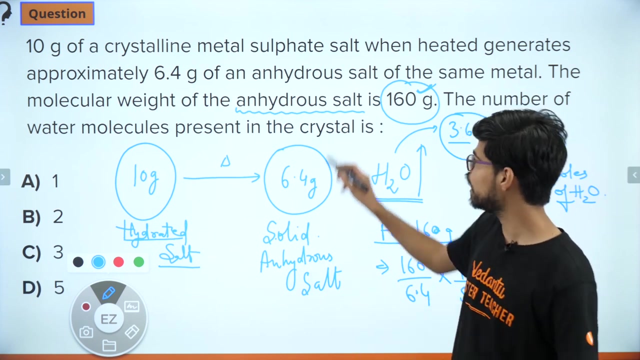 So this is how much? 25, Right. So this will be 5. Okay. so the mistake here is, if you take this 10 grams, here You'll get a different answer. So you'll get 16 by 5 or something else. So anhydrous salt: is this? for 6.4 gram, we get 1 by 5 moles. 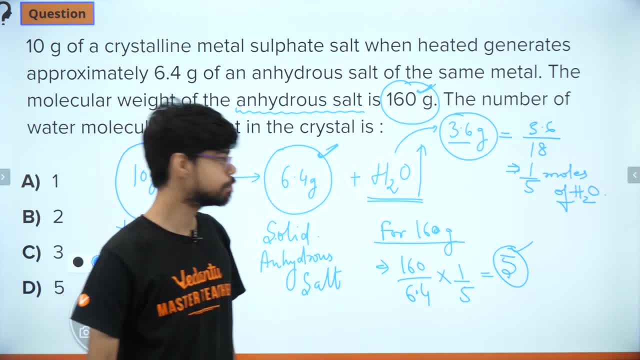 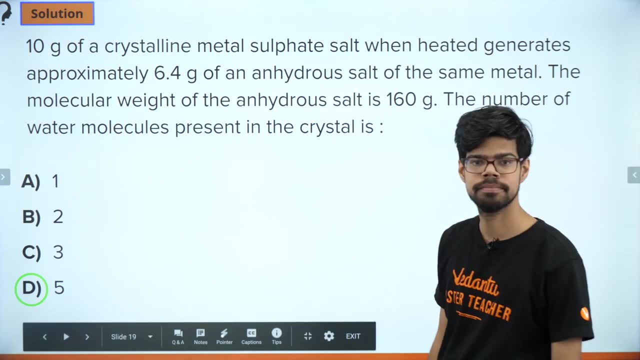 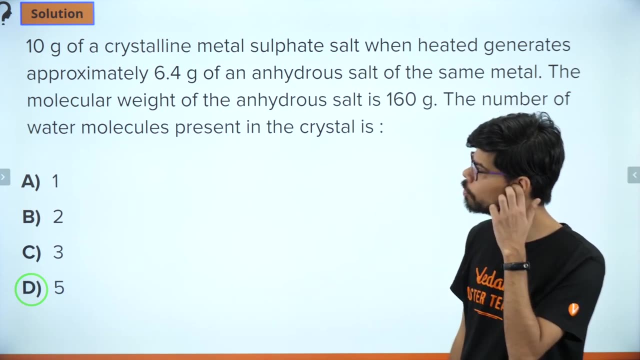 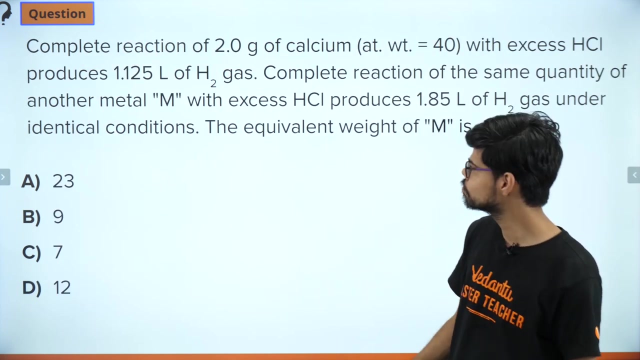 We can calculate for 160 grams. Okay, so answer is 5. Okay, so each crystal or one mole of crystal has five water molecules. This is also a standard type of a problem. You will have seen this many times. What is the next question? I guess this is the last question for today, and this involves equivalence right. 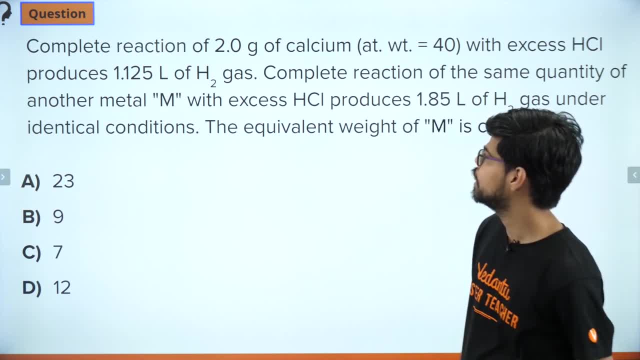 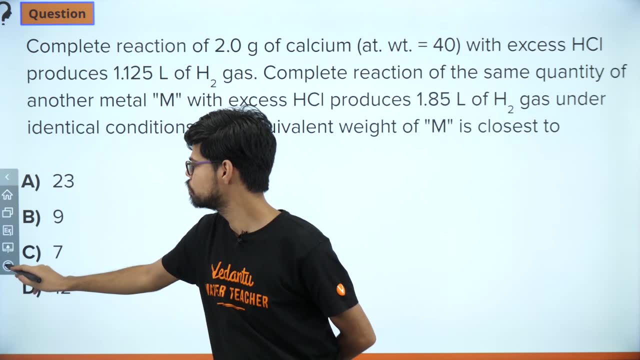 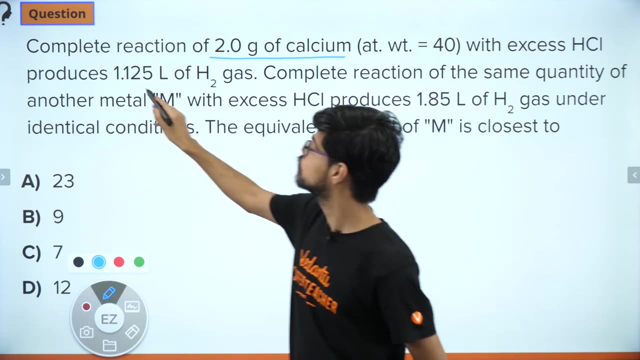 Okay, so let's Do this. What does it say? it says 2 grams of calcium. 2 grams of calcium Reacts with an acid To produce some amount of hydrogen gas. now we will do this problem in a way. We don't have to write any equations. 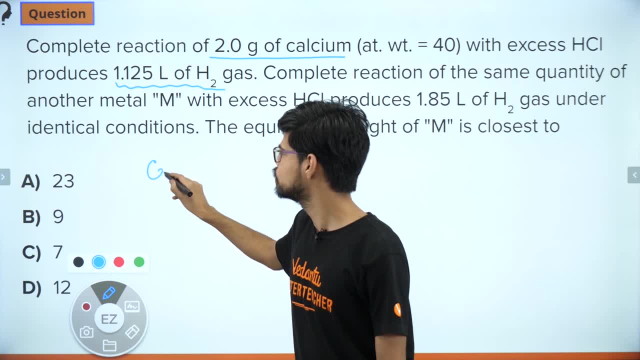 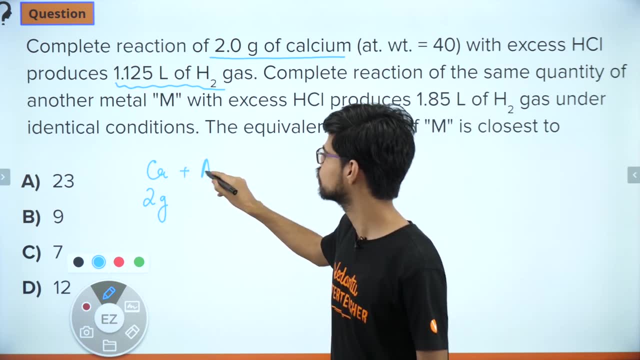 you'll see how, and Just so let me write this. So we have 2 grams of calcium and it reacts with Excess of acid. we have acid, You don't care how much we have excess. So this is the limiting reagent. Calcium is the limiting region. We get some amount of hydrogen. 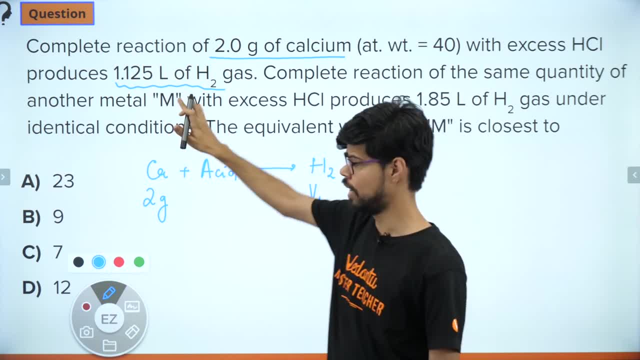 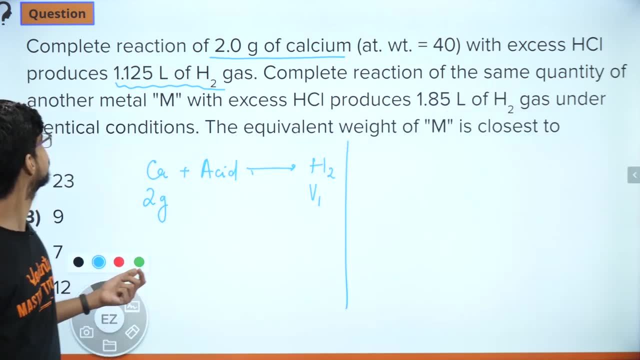 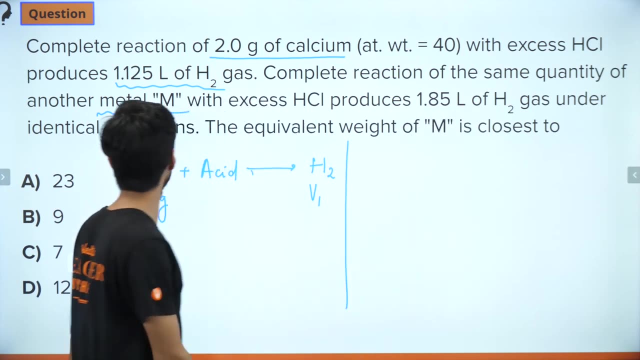 Let's say V1.. Let's write this V1 here, given the value of V1 of hydrogen. now, at the same time, There's another mystery metal, M. right, There's another metal, M, and when same quantity of another metal means 2 grams. 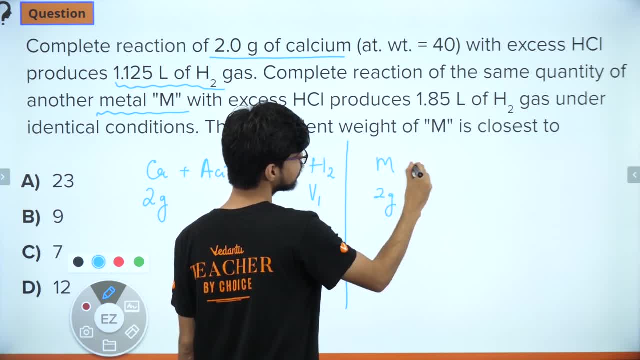 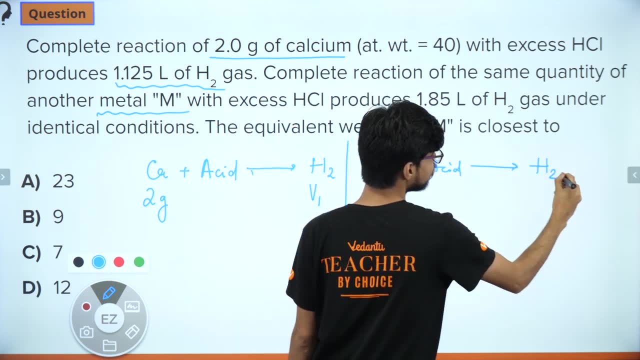 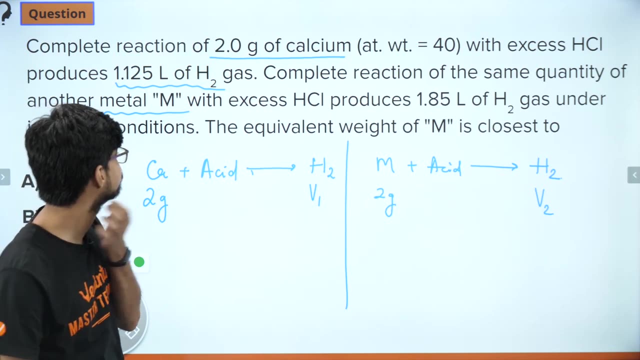 So we have some metal M same. 2 grams of metal reacts with another, same as an excess acid. So the gain: this is the limiting reagent. We get some different amount of hydrogen. Let's call it V2 and it is given as 1.85. 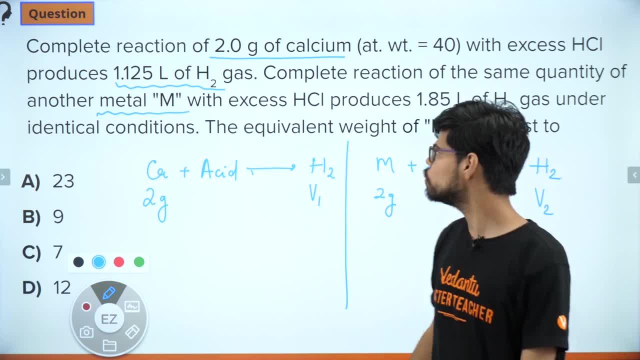 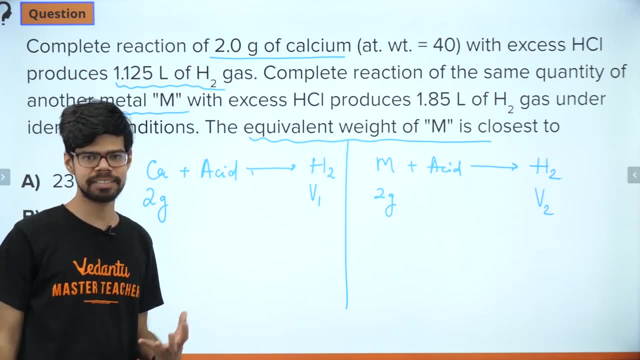 Under identical conditions. so conditions are similar. So you have to kind of equivalent weight of metal and Generally this problem is a little problematic. problematic problem is problematic for class 11 students And you have to understand one very simple thing about this: In the matter of equivalence, what you can say is equivalents. 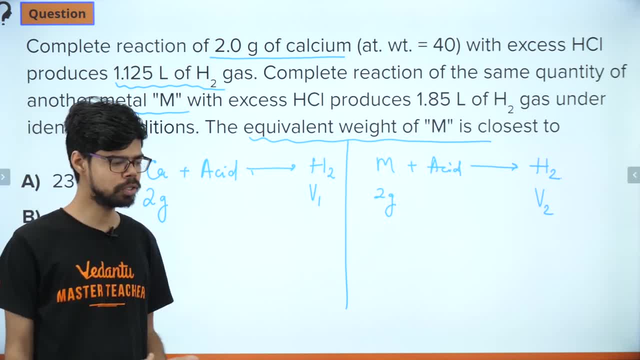 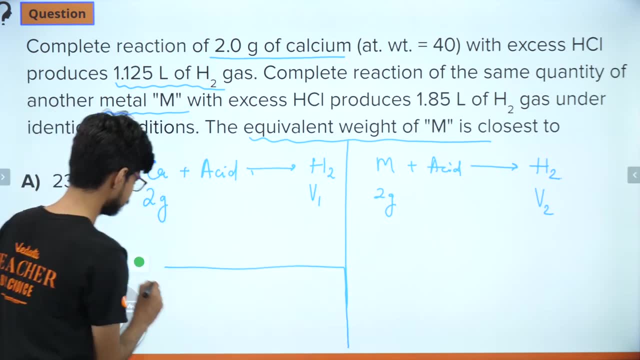 are related to valency. ok, They are related to valency and the molecular weight, And the simple law which you can try and remember is: one mole of hydrogen is released by two equivalents of metal. This is the statement which I have to use. 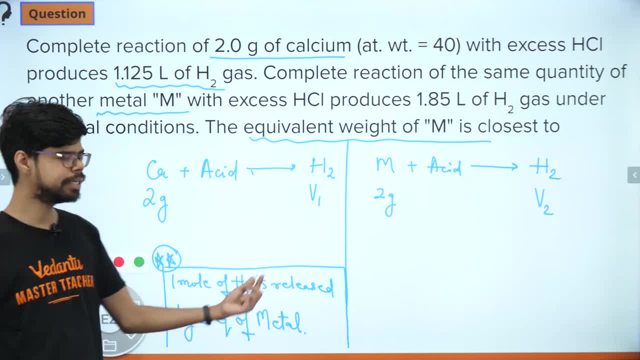 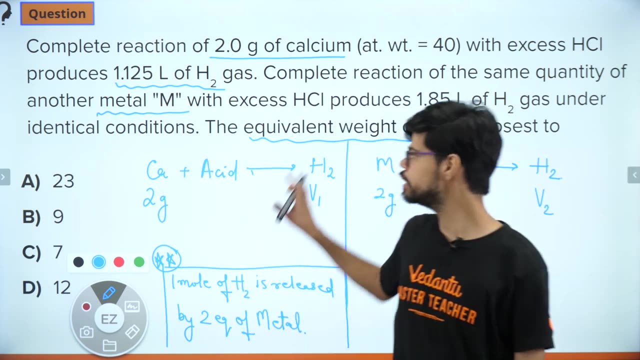 here. So one mole of hydrogen is released by two equivalents of metal. So I can also write it: half mole of hydrogen is released by one equivalent of metal. This is one way to define equivalents for a metal when it reacts with an acid in such a situation. So moles are.